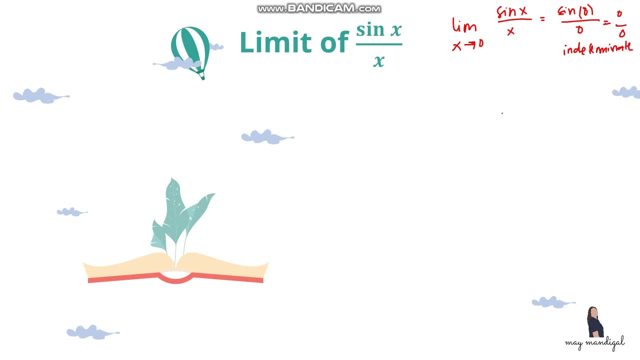 the limit does not exist. Now, if we will go back to the definition of limit, the exact value or the limit of sine x over x as x approaches 0 is equal to 1.. Now you might ask: how did it become 1?? Why not? the limit does not exist. So again, you have to go back to the 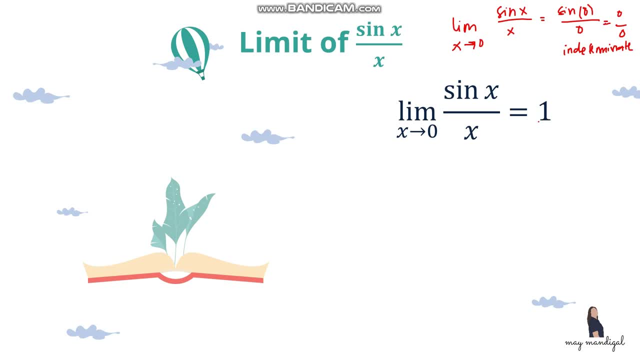 definition of limit, which is, again, this is the value that our function approaches, as x approaches a particular value, or c. So, in order for us to obtain 1, you can use the table of values. You can look at the values on the left side of 0 and also on the right side of 0.. 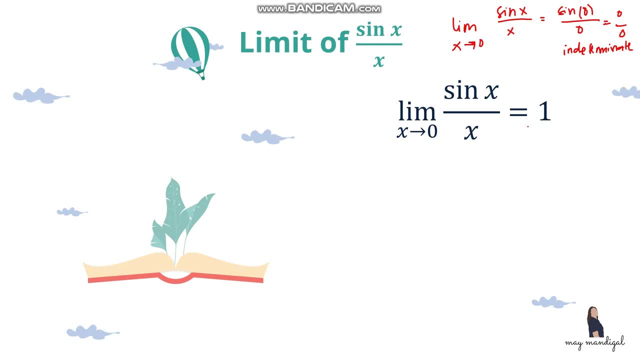 Evaluate the function and notice that those values are both approaching 1.. Another thing that we can use is by looking at its graph. So this is the graph of f, of x equals sine x over x. or this is the graph of our function. Notice that on this part right here, it has a hollow circle. or 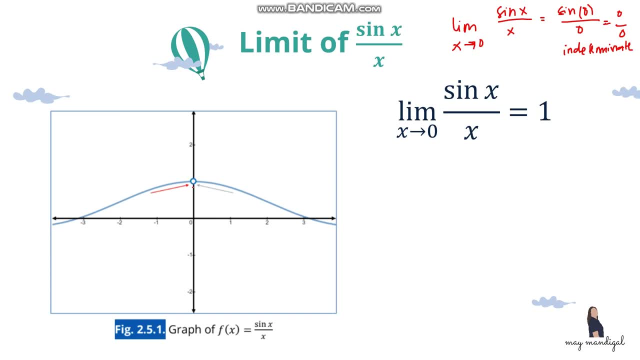 it is a hollow circle. this is where x is equal to 0. So because if we will do direct substitution, like what we did in the first one, so it will be in the middle. So if we will do direct substitution, that means 0 is really not part of the domain. But since we are just talking about the limit, 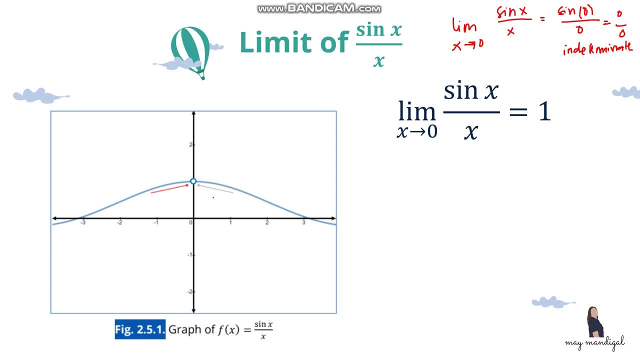 we're not talking about what will be the value of the function if x is 0.. So what I will do is you can look at the graph coming from the left and also coming from the right, and you will notice that they are approaching the same value, which is 1.. That's why the limit of this function. 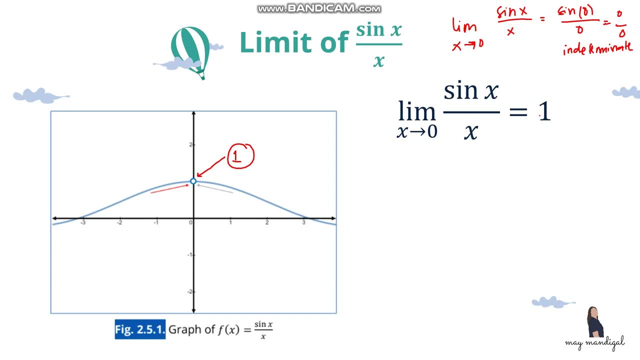 sine x over x. as x approaches, 0 is equal to 1.. That's why it is called a special limit, because, as you can see, if we will do direct substitution, we will get an indeterminate value and we cannot really factor this or do something about this. 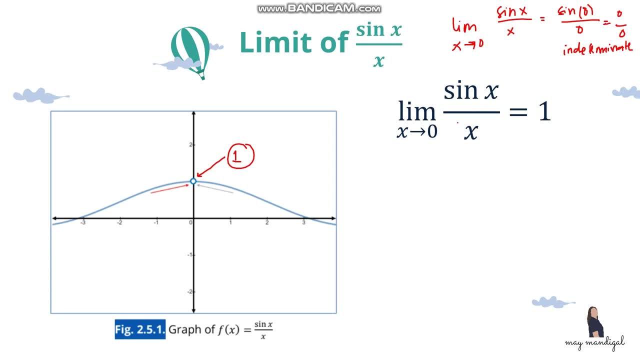 But if we will go back to the definition of limits, we can obtain a value which is again, in this case, is 1.. This is also true for limit of x over sine x, as x approaches 0. So the limit of that is still equal to 1.. Now how will you know if the limit of x over sine x is equal to 1?? Well, you can. 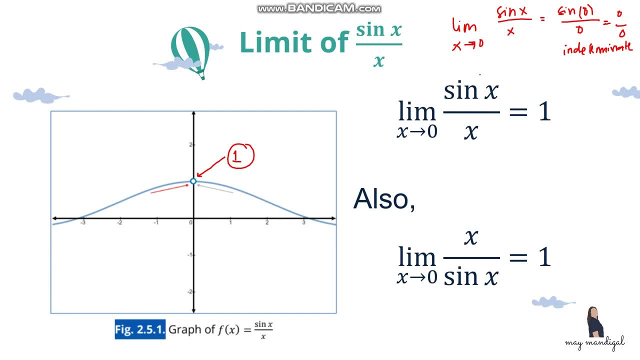 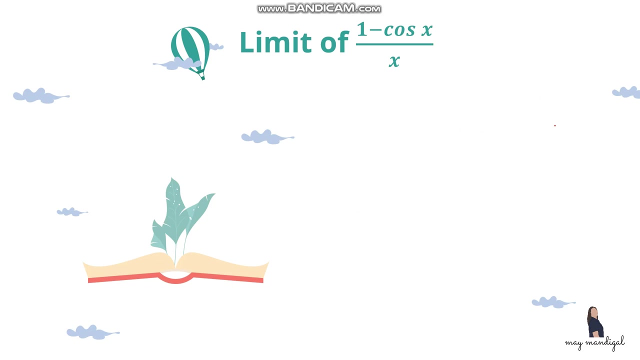 hope that same rule applies here to the finished, unstoppably 거야. quantum кажется avaliable 0, and so you can apply this rule also for the current daily physicalquarters. it becomes indeterminate, automatic. our limit is equal to one. we also have one minus cosine x over x. so, like what we did in the first one, if we will get the 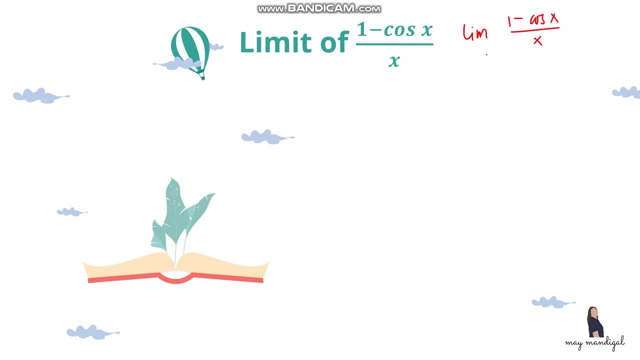 limit of this one minus cosine x over x as x approaches zero. if you substitute zero, it will also be indeterminate. this will happen if you will do direct substitution, but again if we will go back to the definition of limits. this is the value that our function approaches as x approaches. 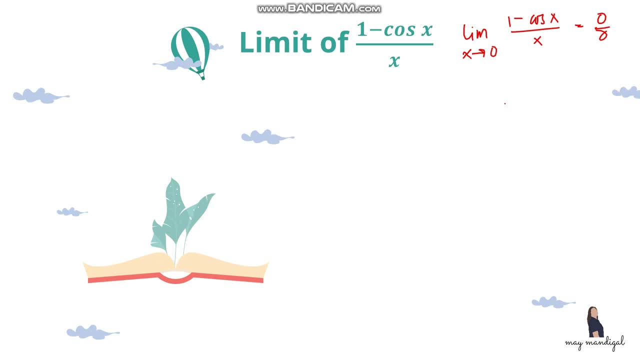 a certain value. so technically, if we will be getting values from the left and from the right of zero, it will approach to a certain value which is zero. okay, and we can also look at the graph. so this is the graph of f, of x equals one minus cosine x over x, or this is the graph of our 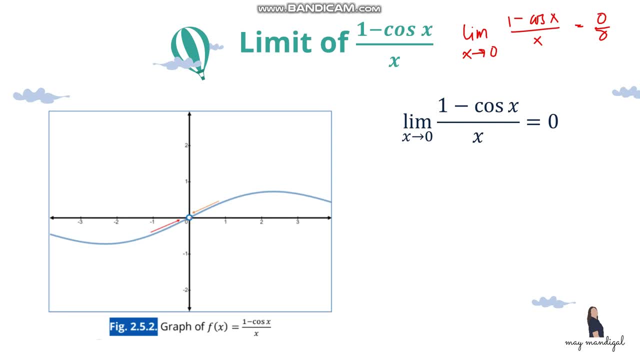 function. notice that if x is zero, there is again a hollow here, which means because if we substitute directly zero to this function, it becomes indeterminate. so zero is again not part of the domain. but if you will look at the graph, see here that as the value of x approaches zero, the graph also approaches zero from left and from. 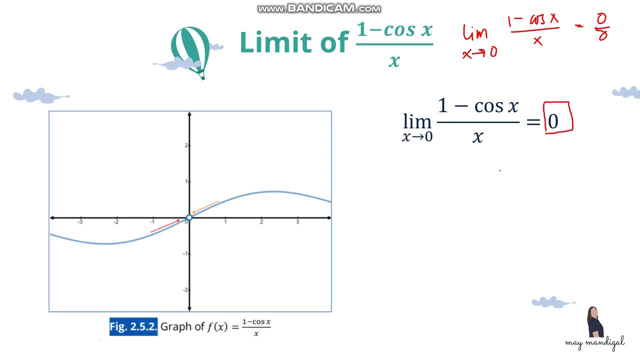 the right. so that's why the limit of this is zero. this is also true for the limit of x over one minus x approaches zero, so that will give us also a zero value. now how will you know if the limit of this particular function is zero? so of course, it should follow this form: one minus cosine x over x. 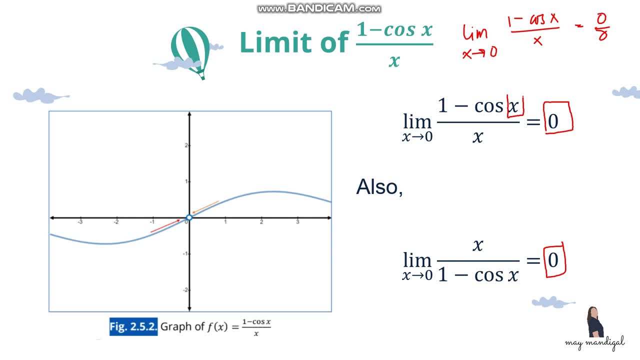 now the value here. so the function of the cosine must be the same with the denominator. so that is your indicator, one of the indicators, so that we can say that the limit of it is zero. and if you substitute this c to your function, it should be indeterminate, and if that happens we can directly 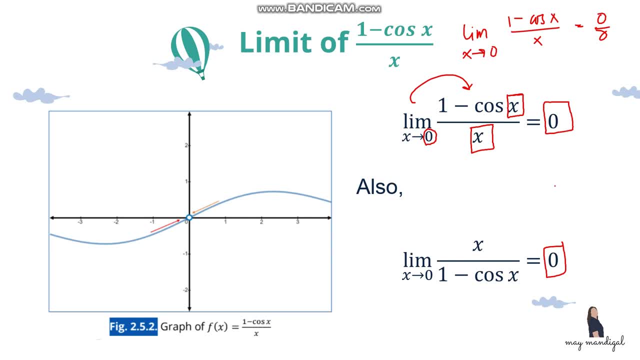 say or conclude that that limit of the function is zero. so as long as the function of the cosine and the denominator are the same and when you substitute c to that function it will become indeterminate automatic. the limit of that is zero. and for the last one we have limit of e raised to. 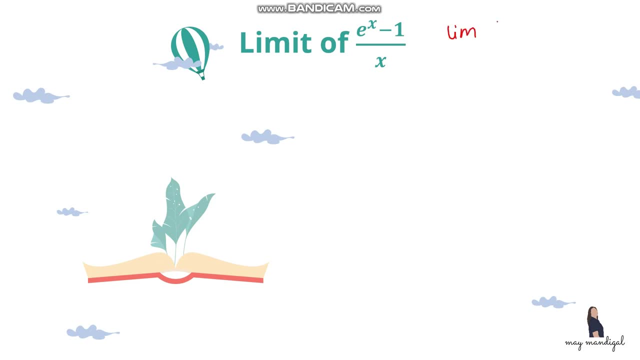 minus one over x. so again, if we solve for the limit of that as x approaches zero, so this will become e raised to zero, or one minus one over zero, so that will be zero over zero or again indeterminate. so we cannot do anything about this, we cannot simplify this. so 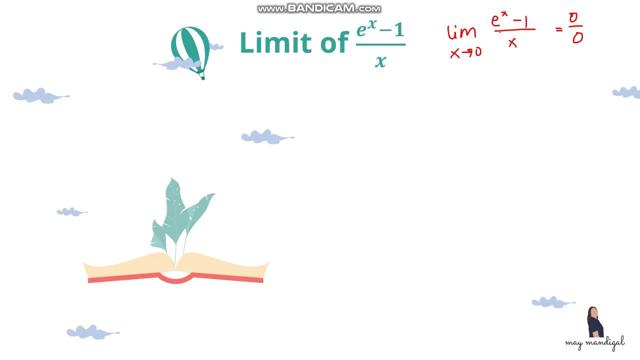 we can use the table of values again, and also the graph, to see the actual value of the limit of this function. now, if you do that, we will obtain a value of one. so that means if you get the value from the left side of zero and also from the 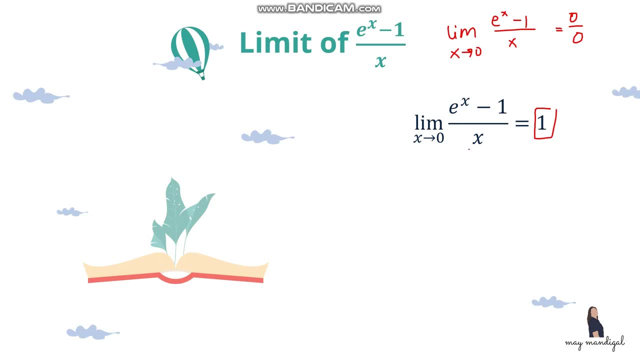 right side of zero, all of them will approach the value one if we will look at the graph. so this is the graph of e of x. so this is the graph of e raised to x minus one, all over x. again there's a problem because if you substitute directly to our function, it's indeterminate, but as the value of x 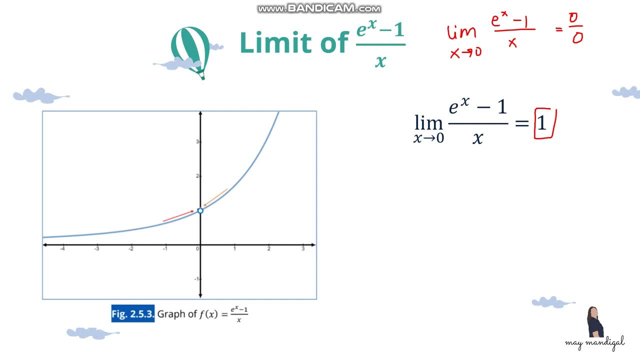 approaches zero, the graph of the function from the left and from the right approaches this value, which is one. so this is also true if we will have limit of x over e raised to x minus one. as x approaches zero, still it's equal to one. so again, when can we say that we can apply this value? 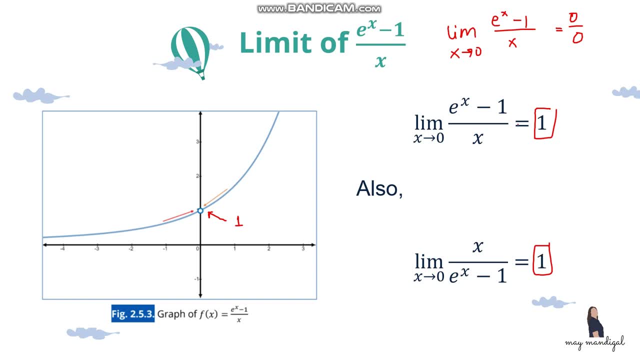 for the special limit. so if it follows this form, e raised to x minus one over x, or as long as the exponent of e is the same as with the denominator, and when you substitute c to that function it becomes indeterminate, then that means the limit will still be equal to one. so for the general steps. 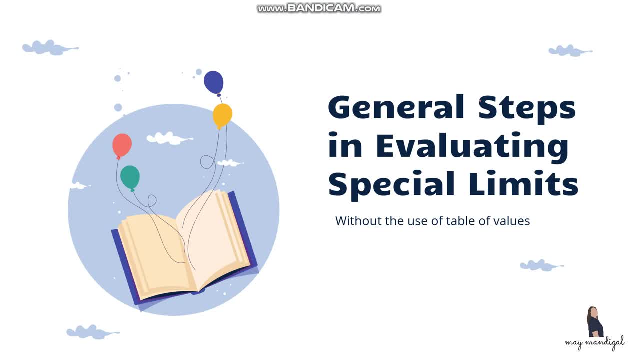 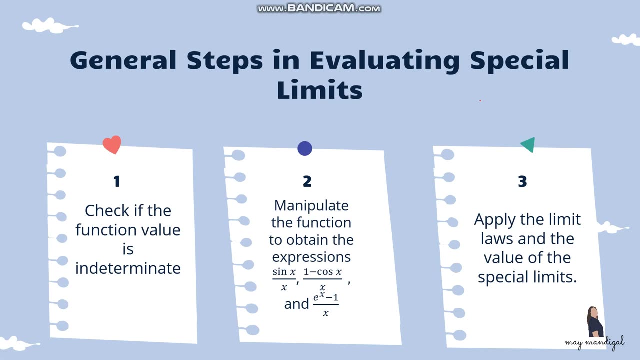 in evaluating special limits, of course, because we will not be using table values all the time. also the graph, because of course we don't want to waste a lot of time in substituting and evaluating using the table of values. so here are just some of the general steps that we can do. so first is check if the function value is indeterminate. so this is: 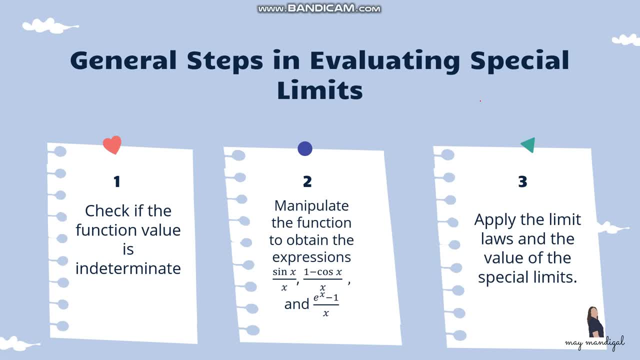 the first thing that you have to do, so substitute c to the our function if it becomes indeterminate. so we have now to go to the next step, which is to manipulate the function to obtain the expressions sine x over x, one minus cosine, x over x, and e raised to x minus one all over x. so, after checking if it's indeterminate, we now have to 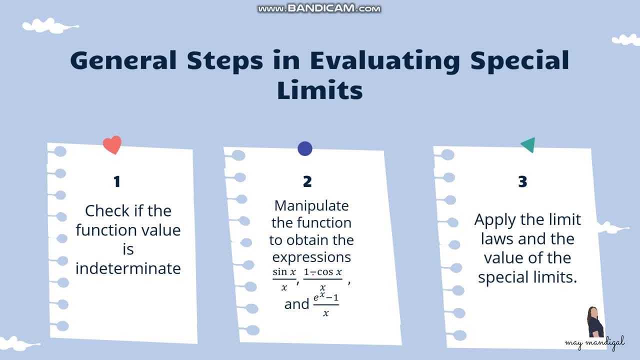 manipulate our function in order for us to arrive in any of these three expressions. once we already have these expressions, then we can now apply the limit loss and also the value of the special limits. again, as long as the sine or the function of sine is the same as with the denominator, the function of the cosine is the same as with the denominator. 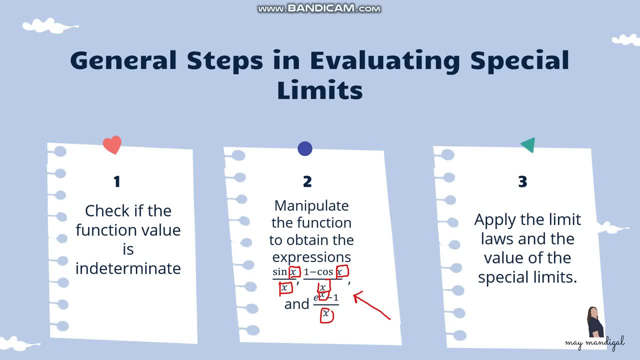 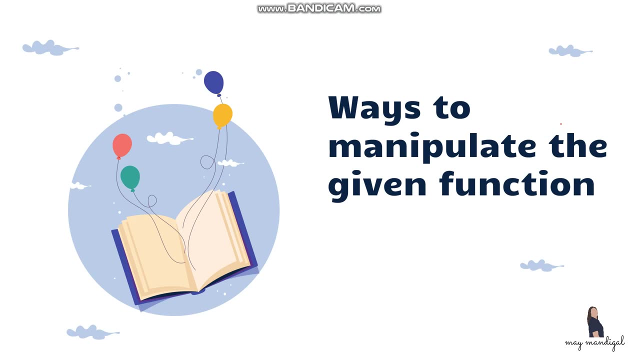 the exponent of e is the same as with the denominator, and when you evaluate them with the value of c, it becomes indeterminate. then you can apply the value of the special limits. now, what are the ways to manipulate the given function? so here are just some of the ways that. 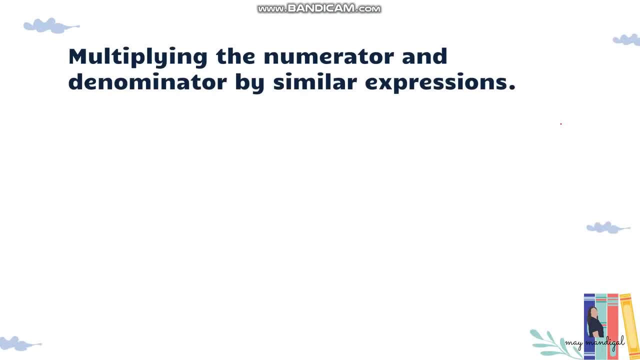 we can do first is we can manipulate by multiplying the numerator and denominator by similar expressions. so, of course, if we want to arrive at a particular uh format, so we have to manipulate it, so we have to manipulate it, and one way is by multiplying the numerator and denominator by similar expression. 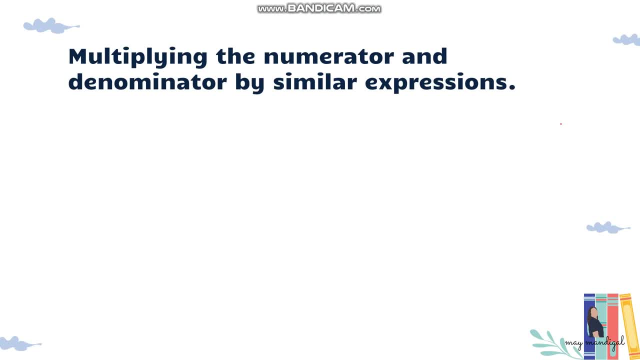 remember, the number that you will multiply on the numerator must also be the same with the one that you will multiply in the denominator, so that we can just retain the value of the function itself, because multiplying the functions by- uh same numerator and denominator, it's just like you're multiplying by one. 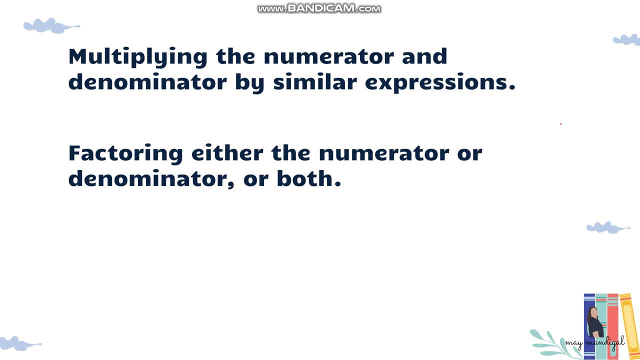 another one is factoring either the numerator denominator or both. so another step is we can factor if the terms are factorable. so either the numerator denominator or both. and then, after we factor, we simplify it even more. and last, we can do splitting of the fraction as the sum difference. 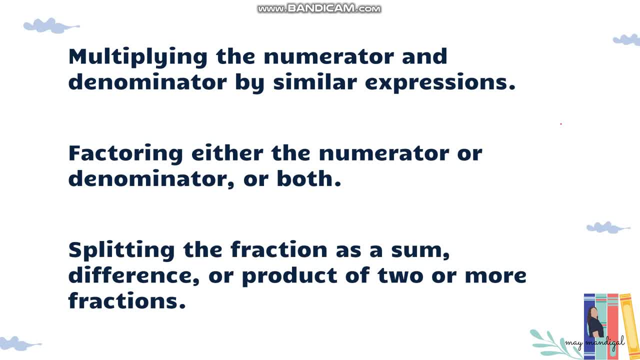 of the product of two or more fractions. so later you will see if you think we can write them separately into two or more different fractions, then we can also do it. so these are just some of the ways on how we can manipulate our function. so let's start with this example. let's say we 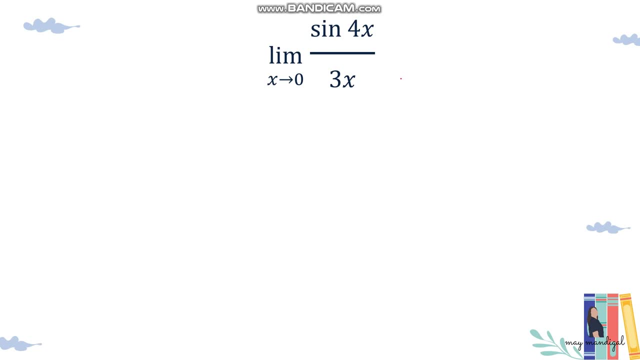 have to identify the limit of sine 4x all over 3x. so first step that we have to do is two check. if this will be indeterminate, if we substitute 0, so that will be sine 4 times 0 over 3 times 0. 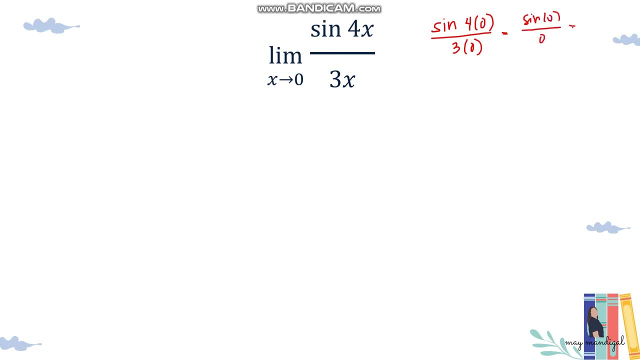 this will give us sine of 0 over 0, or again, this one is indeterminate. now, after checking, since we identified that it is indeterminate, we now have to manipulate our function and notice: um, we have. so let's just write here first: sine 4x over 3x. okay, now we have to go back to the forms, the three. 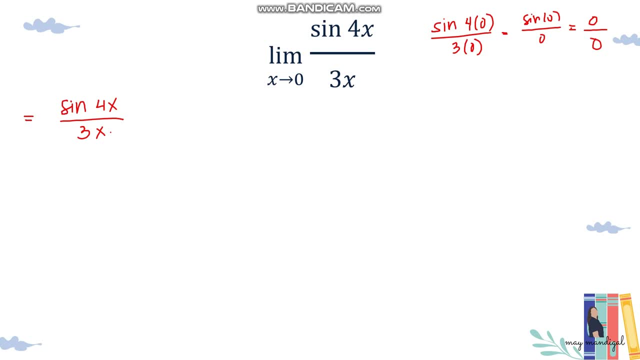 forms that I showed you a while ago: the one with sine, the one with cosine and then the one with the e or the natural number. so you have to think: which among the three do you think is possible for us to obtain in this given function. so since we already have sine here, that means we have to arrive at 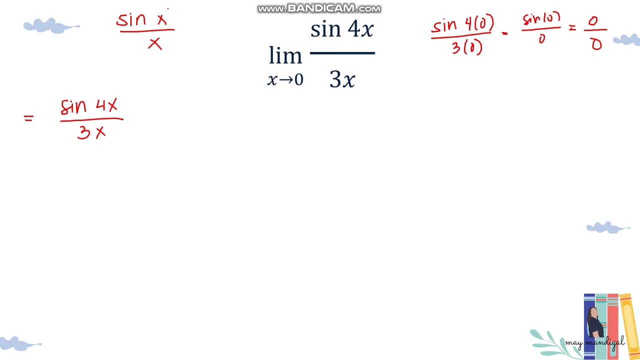 sine x over sine x later on. but again, it's not always x here and x as long as they are the same. so, um, everything will still be applied. so we have to make now 4x and 3x here the same. now, how are we? 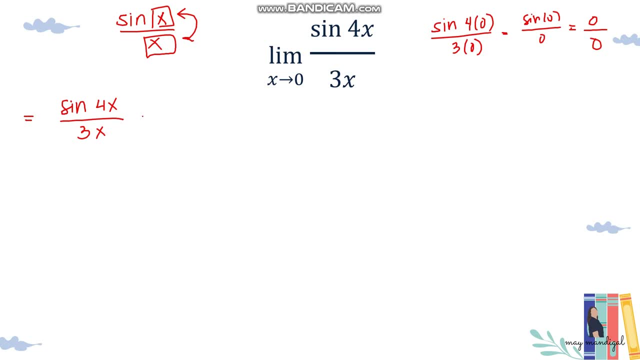 going to make them the same same number. so let's go back to the techniques. so we can multiply, we can um um factor, or we can split. so we cannot split this into fractions, because um sine 4x is just one term. we cannot factor because it's already in simplified form. so what's left for us is multiplying. so we 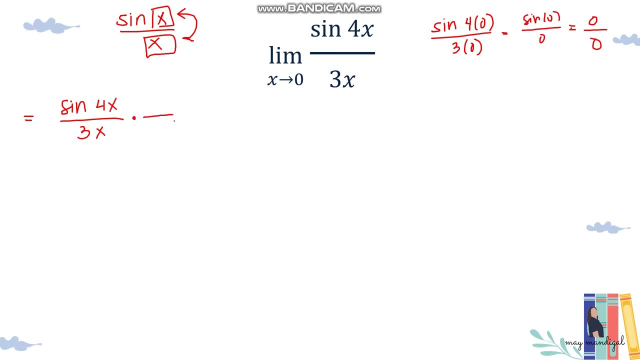 have to multiply now. now, in multiplying you have to think what number should we multiply so that when we multiply it we can arrive with our goal? so our goal is to make them the same number. now just a tip, if you want to make them the same number for you to easily identify: what number will you multiply here? 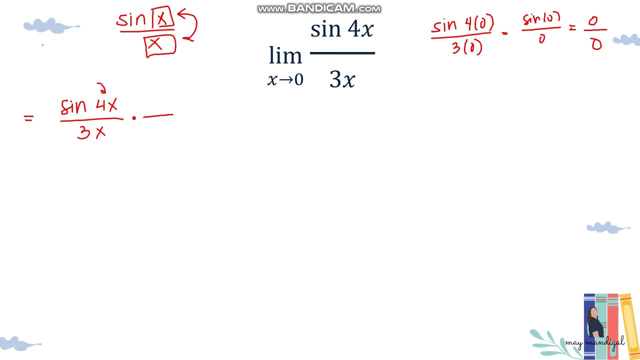 so you focus with the numerator. so what we have there is 4x. so let's write here sine of 4x. now, since 4x is part of sine, because it's sine 4x. that means it's a bit difficult, if we will try. 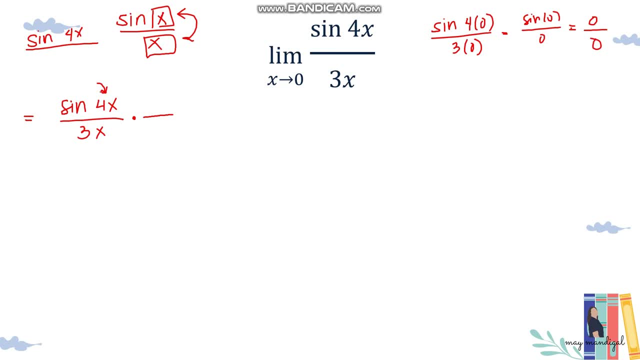 to make it into 3x. so what we will do is we will focus with the denominator and our goal is to make into 4x. okay, so our goal now is to make this 3x, transform this into 4x. now, how are we going to? 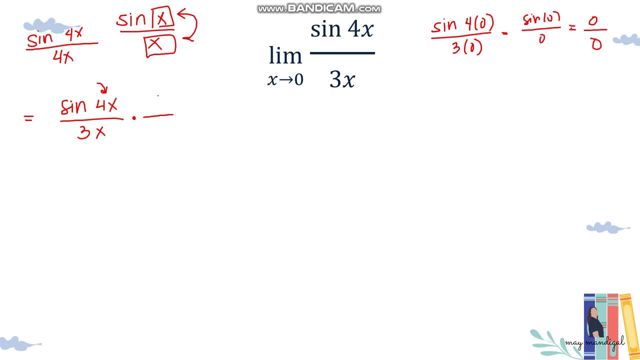 transform this into 4x by multiplying a particular number. since this is our goal, what you can do is you can just get the numerator and then that's the number that you will multiply here. okay, so we can have here 4 over 4. so this is just one way on how you can multiply a number. you can think of other. 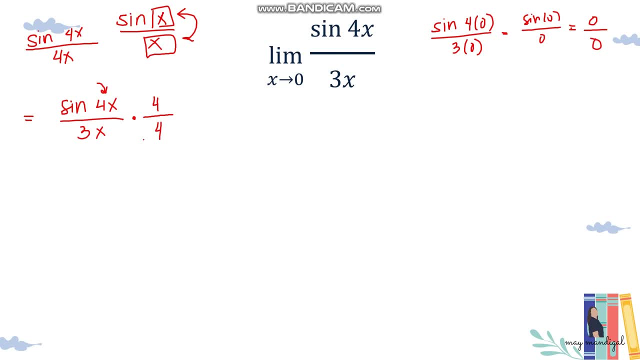 numbers to multiply as long as you will arrive at 4x in the denominator. so again, what we did is we just get the numerator, whatever the coefficient of x here, that is the one that we will multiply, both numerator and denominator, and then let's multiply. but what we will do is we just write. 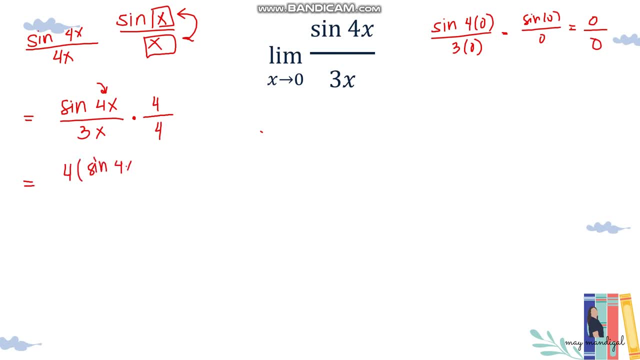 them together, so 4 times sine 4x, 4x, 4x over, and then what we have here: 3x times 4, so that is just 4 times 3x. now again, our goal is to make our denominator equal to 4x, but since we already have here 4, 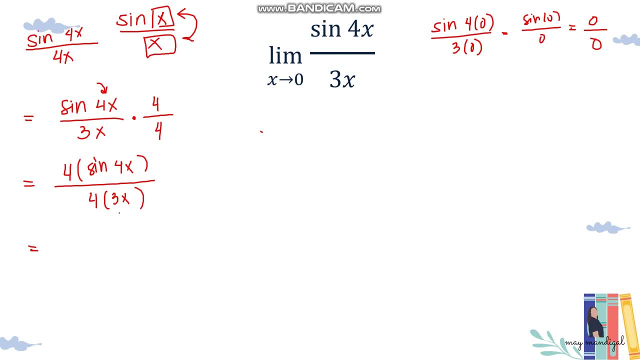 times 3x, since this is multiplication. so that means we can interchange the values or the, the numbers, and we will still have, or we will still arrive at, the particular value, which is, if we multiply this, we'll still get 12x. so what we will do is you have 4 times sine 4x and then to have 4x. what we will do is we will. 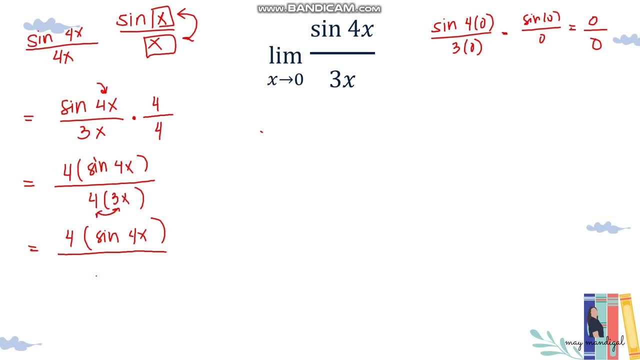 just change 3 and 4, so we will put out 3 here and then we will move 4 inside the parentheses, so we have here 4x. okay, so by just changing the grouping symbol or by interchanging the values, we're able to obtain 4x. 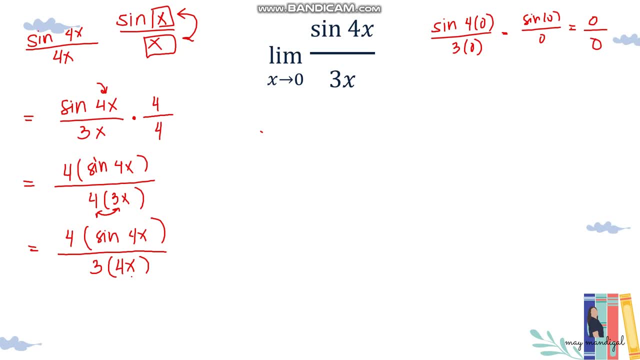 so if you multiply this 3 times 4x, still it's equal to 12x, so nothing changes. okay, so now we have sine 4x over 4x, so we're able to arrive at our goal, which is this one. so what are we going to do with 4 3rds? so we just have to write them in a separate fraction. 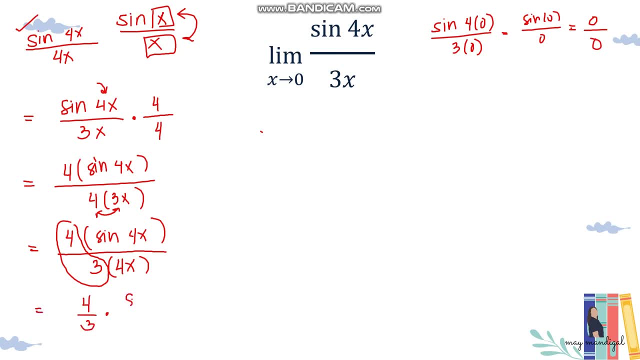 so that will be 4 over 3 times, then sine 4x over 4x, now after that, once we all already achieve our goal. so we will now identify the limit. so let's write here limit of and then let's just close it in a grouping symbol like this: times: sine 4x over 4x as x approaches 0. now. 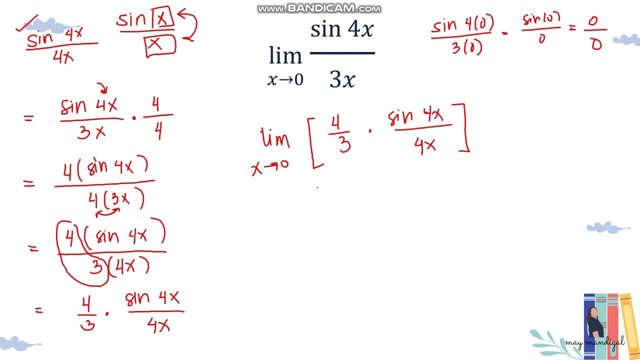 what we will do is we now have to evaluate the limit of this. so you have here limit of 4 over 3, so that is just 4 over 3 times. and then how about? for this one? it's now sine 4x over 4x. okay, so, like what i've said, a 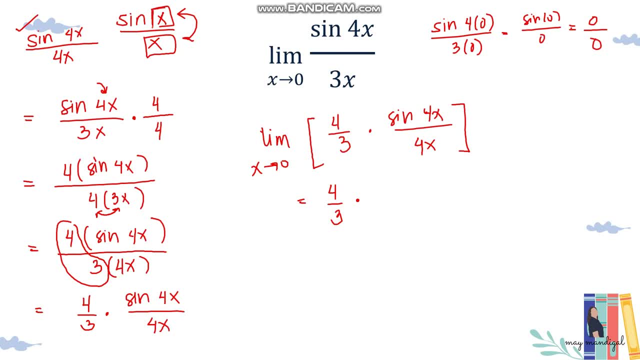 while ago. as long as the function of x is the same as with the denominator, then the property for the or the value for the special limit is still applicable. but we have to make sure that if we substitute the x here, it will be indeterminate. so since c is 0, if we substitute 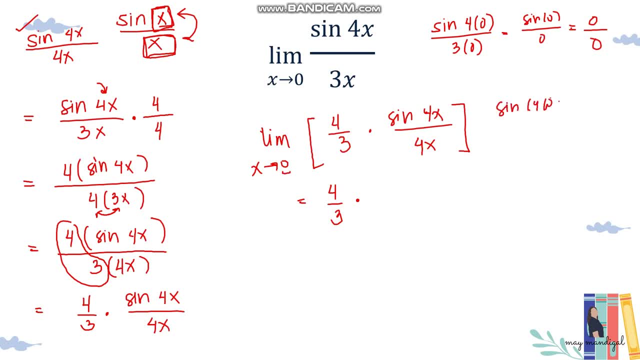 here it will become 0, and then we have to calculate the value of x, and then we have to calculate the sine 4 times 0, over 4 times 0, which is still indeterminate, since it's indeterminate and at the same time function of the sine. here and the denominator are the same, they are both 4x. 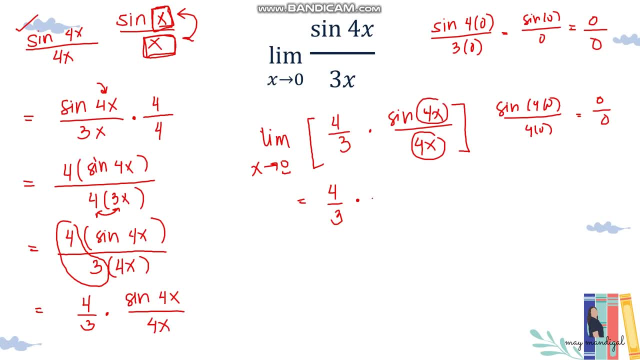 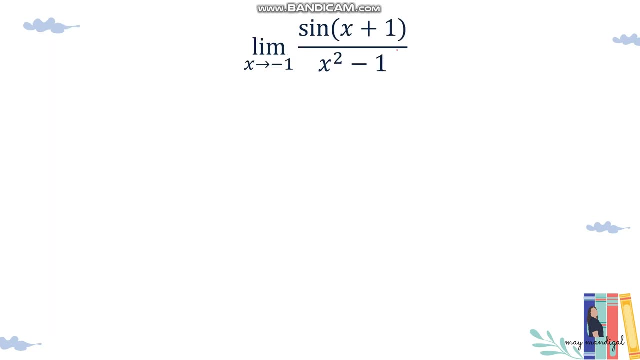 therefore, we can still say that the limit of this function is equal to 1. okay, so it will still hold true for this given example. so simplify that. so we have 4, third, as our limit. so we have here limit of sine x plus 1 over x squared minus 1 as x approaches negative. 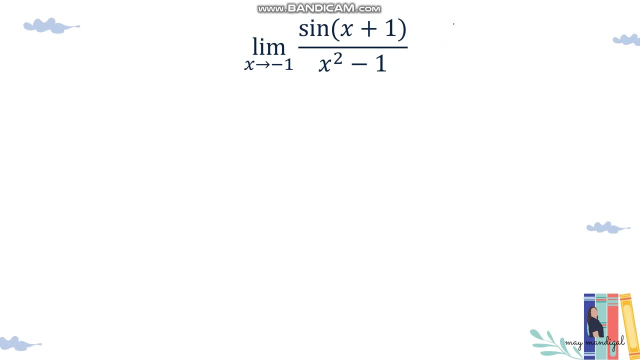 1. so if we substitute that sine negative 1 plus 1 over negative 1 squared minus 1, this will again give us an indeterminate value. so that means we cannot do direct substitution. so let's check: what can we do with this? so sine: 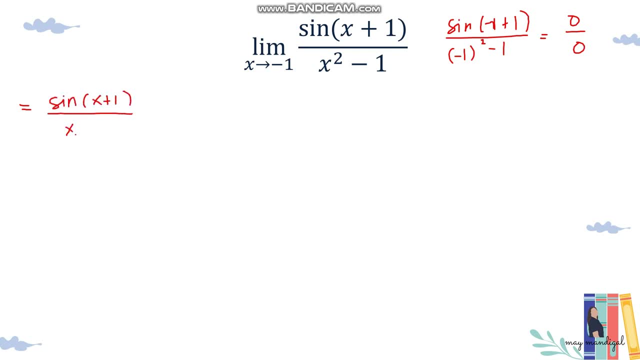 x plus 1 over x squared minus 1. okay, now again observe. observe the function that we have. since we have here sine, that means we can use the first form, which is sine x over x. so we should arrive at something like this later on, but since what we have here is x plus 1, therefore, our goal is to 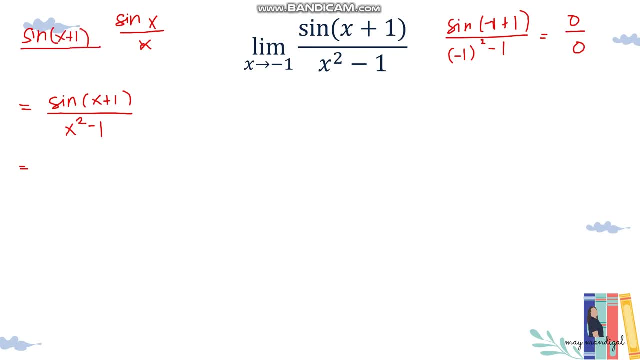 arrive at sine x plus 1 over x plus 1. so this is our goal. so we should arrive at this point. now what can we do with our function? as you can see, the denominator here is x squared minus 1, so that means we can try factoring the denominator so that. 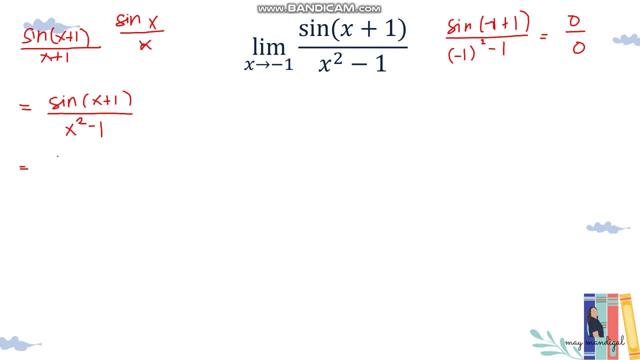 we can have x plus 1 here. so let's try sine x plus 1 over and then factor out x plus 1 times x minus 1, our denominator. so it's x plus 1 times x minus 1. now, as you can see here, after factoring we're able. 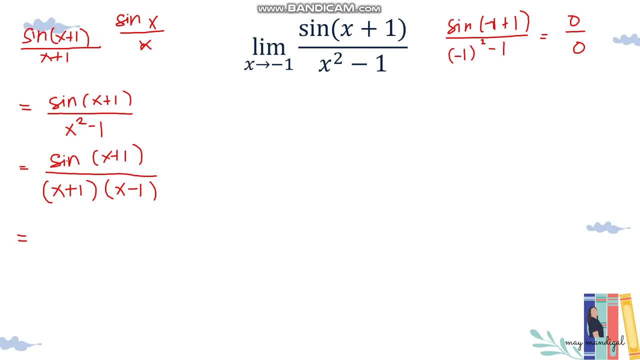 to identify now this function: sine x plus 1 over x plus 1. so this one right here there, so we can write it separately. so we have sine of x plus 1 over x plus 1, so we're able to get now the function that we want: times. how about this? we have x minus 1 in the denominator, so we just have to. 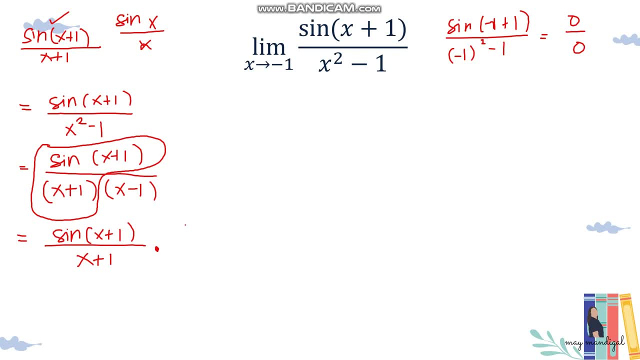 put it out of the fraction and then write it separately, so that will be 1 over x minus 1. so we're able to arrive at our goal, which is again this function right here. so that means we can now write the limit. so limit of. then let's write here sine x plus 1 over x plus 1. 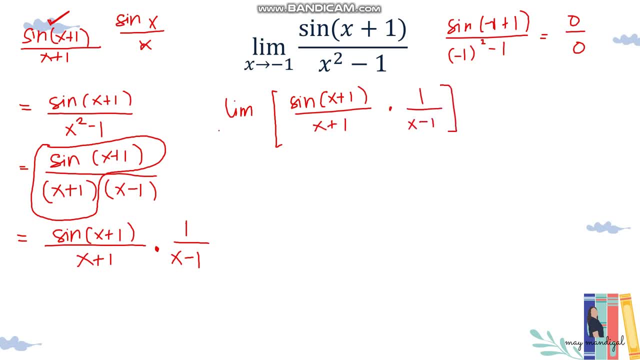 times 1 over x minus 1, as x approaches negative 1. okay, now let's identify the limit of this function. you might be wondering: uh, what are we going to do this time? x approaches negative 1, but a while ago everything approaches 0.. so is it still applicable or is the values of the special 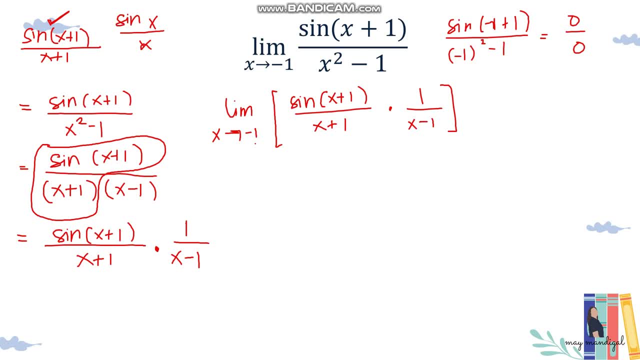 limit still applicable. so let's check again. uh, what we have here is that the function of sine is the same as with the denominator, so we already satisfied one of the condition. another thing is that when we substitute c to this function, it should be indeterminate. if that's the case, if it becomes indeterminate, 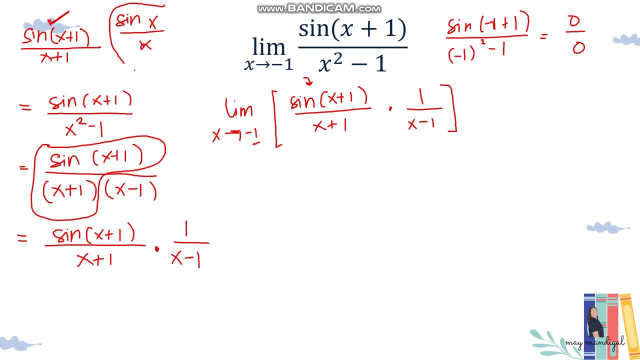 that means we can still apply the special, the value of the special limit of 4 sine x over x. so let's check. so sine negative 1 plus 1 over negative 1 plus 1, so this will be sine of 0 over 0 or still indeterminate. 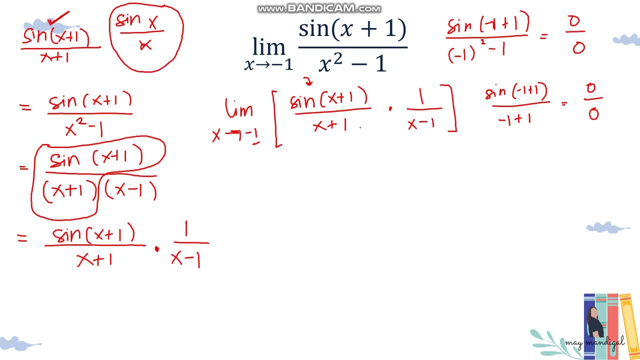 if it happens that this is indeterminate, therefore, we can again apply the special or the value of the special limit for sine x over x, which is equal to 1, and then for the other limit. so we just have to substitute, so 1 over negative, 1 minus 1, so we have here 1 times 1 over negative. 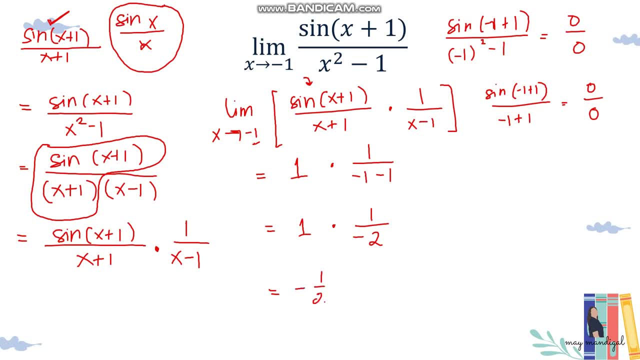 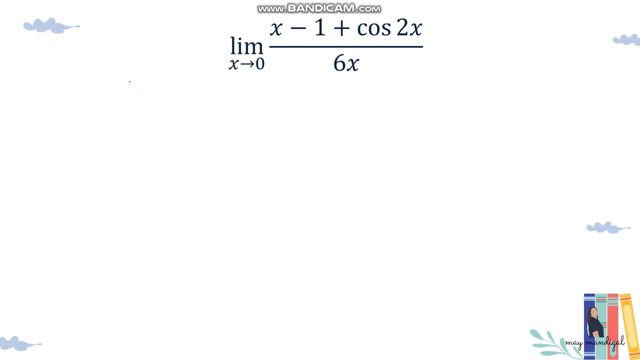 2, or our final answer is negative one half. so this is now the limit of our function. another rule of thumb is that we need to do something to eliminate the limit of our function. so let's say we have limit of x minus 1 plus cosine 2x, all over 6x as x approaches 0. so 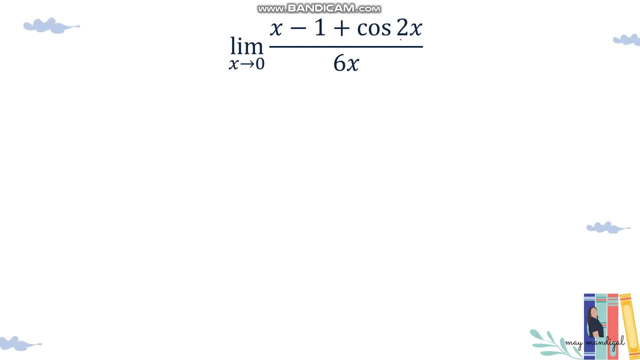 if we substitute 0 here, it will become indeterminate. so you have 0 plus, you have 0 minus 1 plus cosine of 2 times 0 over 6 times 0. that will still give us an indeterminate value. now how are we going to manipulate this? 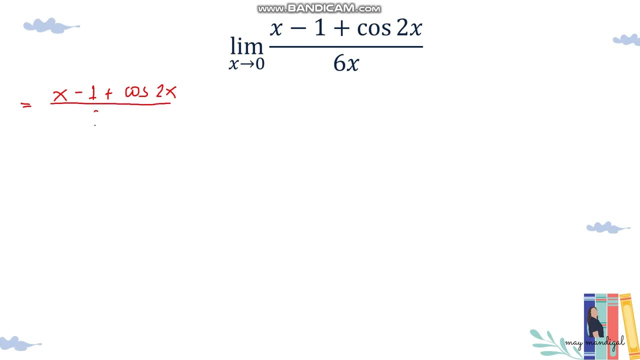 the limit of this function. so for our techniques or the ways on how to manipulate, you can multiply. i don't think it is advisable to multiply it right away. so let's scrap the concept of multiplying factor. we cannot factor here, so the last thing that is left for us is splitting into different. 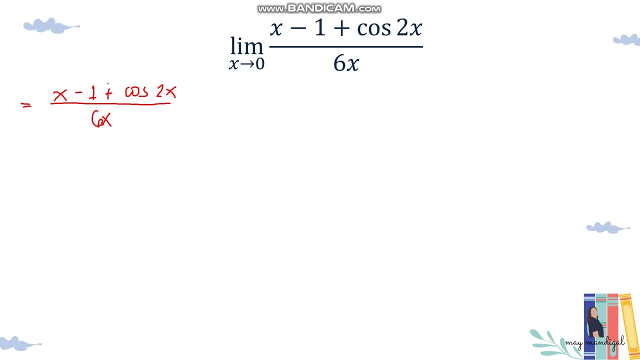 set of fractions. so how are we going to split this into fractions? so you have to look first what uh form are we aiming here? is it the one with sine, the cosine, or e? so since what we have here is a cosine, that means we are aiming to have one minus cosine of x over x, or something in this form. 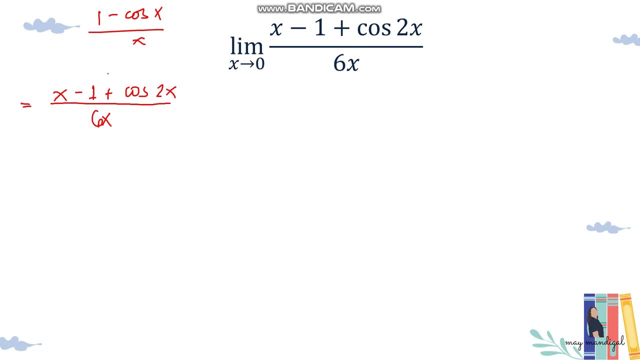 so when you divide this or when you split this into set of fractions, so you have to consider that you should get something like this, okay. so let's try it with this one. we can take this x and 6x and we can write them as one fraction. so let's write here: equals x over 6x, and then plus, and then the. 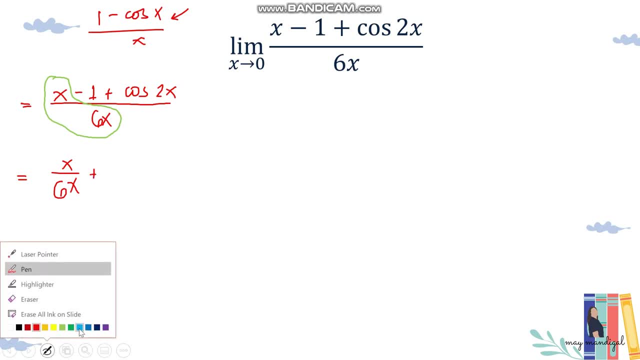 remaining terms. let's write it in one fraction also, so this one negative one plus cosine 2x, all over 6x. they just share the same denominator here, so let's write negative 1 plus cosine 2x over 6x. now let's just fix this. 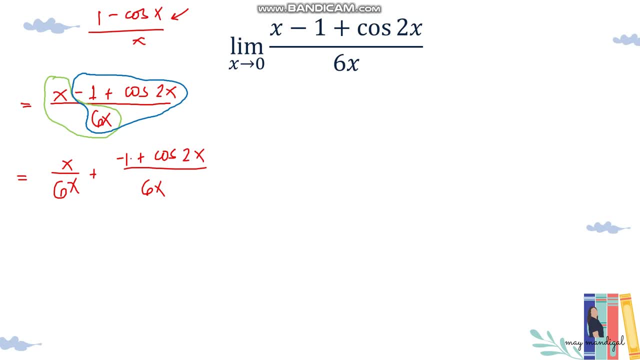 since in the original form it's minus and then this one is plus. what we can do is we can factor out the negative one and then write this as x over 6x, plus negative, then 1 minus cosine, 2x, all over 6x, and then let's just change this, since this one is positive. 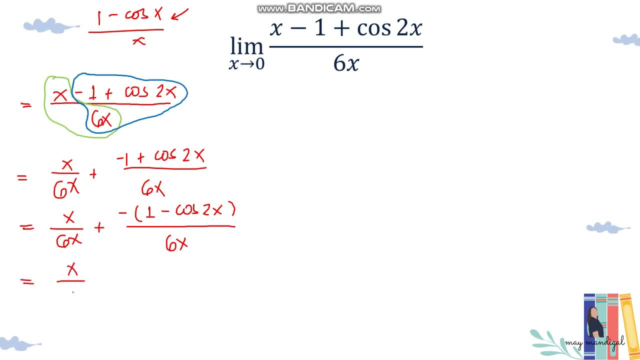 negative, so it will become negative here. minus. then we have 1 minus cosine, 2x over 6x now after fixing the signs. so we now have this, something like this. so what we will do is we have to make them similar, the two here, the 2x and also 6x. we have to make them the same. now, how are we going? 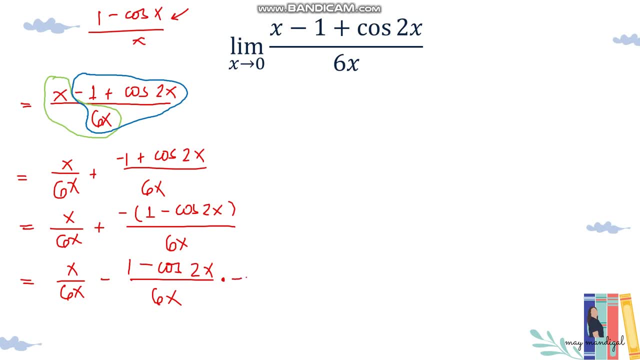 to do it so we can multiply by a number. so remember the technique that we used a while ago in the first example: if you want to make the numerator denominator the same, just look at the numerator. so in this time it's a function of cosine. you look at the numerator and then take. 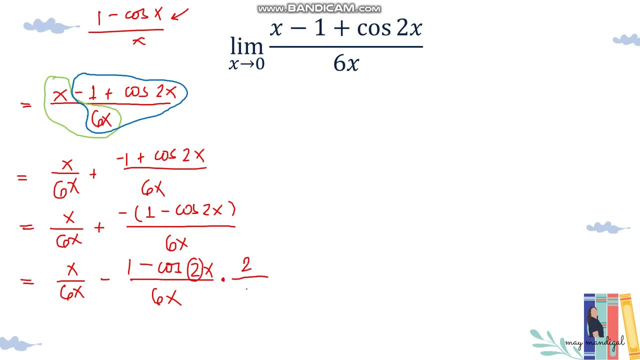 that number and then multiply it, both the numerator and the denominator. so let's do the same thing here. so this will become, by the way, this will be cancelled, so that will be 1 over 6 minus. and then let's multiply, so you have 2 times 1 minus cosine 2x. 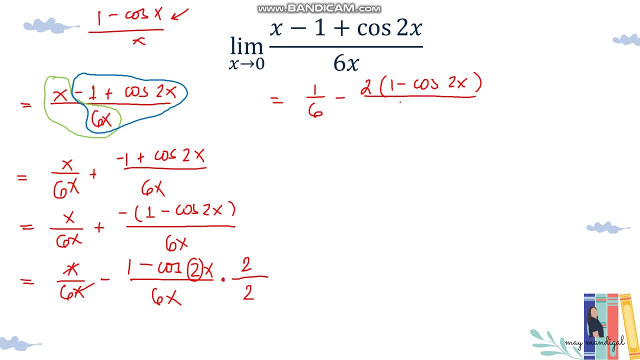 over. and then we have here 2 times 6x and same as what we did in the first example. all we have to do here is to change 2 and 6, so this will become 1, 6 minus, and then 2 times 1 minus cosine 2x all over. let's interchange the 2, so we have here 6 times 2x. so 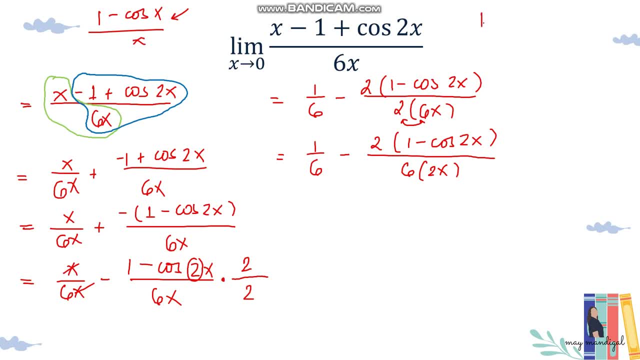 there we now have this form: 1 minus cosine, 2x over 2x. okay, so we're able to get something like this. now we have to factor out 2, 6 or 2 over 6, so that will be 1, 6. 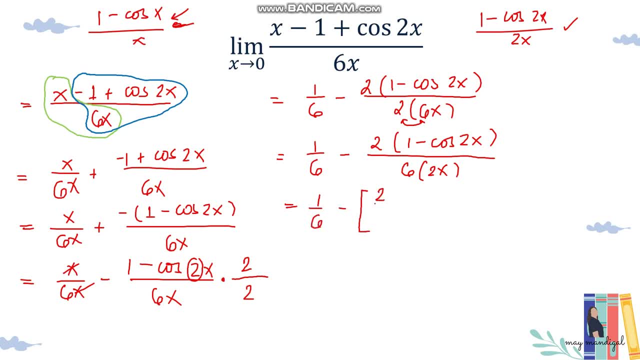 and let's try to put some brackets here: 2 over 6 times, then 1 minus cosine 2x, all over 2x. okay, now that we already have this function right here, following this form, we can now proceed with evaluating the limits. so limit of then we have 1 over 6 minus 2 over 6 times 1 minus cosine of 2x. 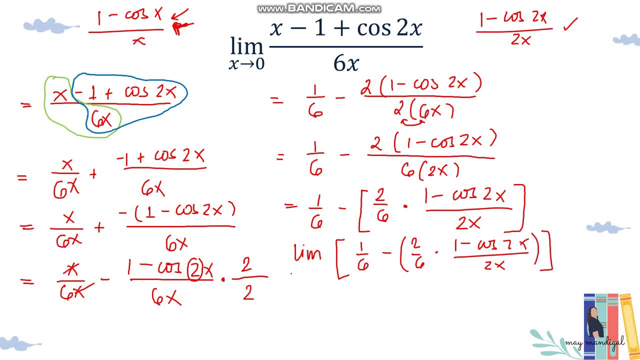 all over 2x as x approaches 0. okay, so 1 over 6 is just 1 over 6 minus, and then we have the 2 over 6 here. now how about this? so this is 1 minus cosine 2x, all over 2x, so they have the same. 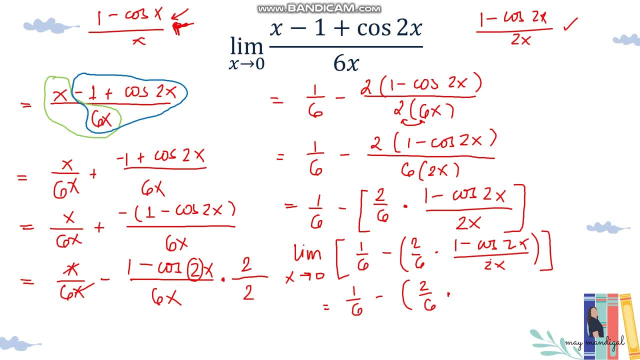 so numerator and denominator. if you substitute 0 to it, it's indeterminate. so that means we can still apply the same value for the special limit of the cosine. so that is 0, so this one is 0, and then you simplify this. so what we will get here is: 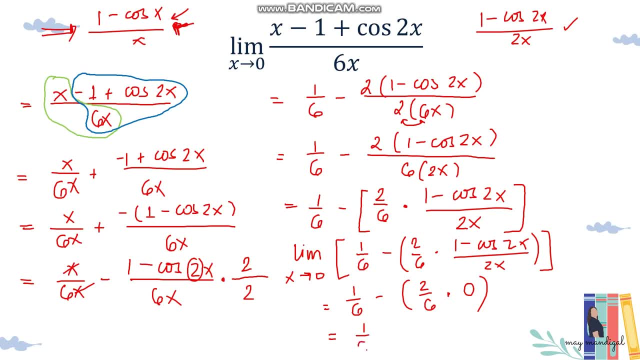 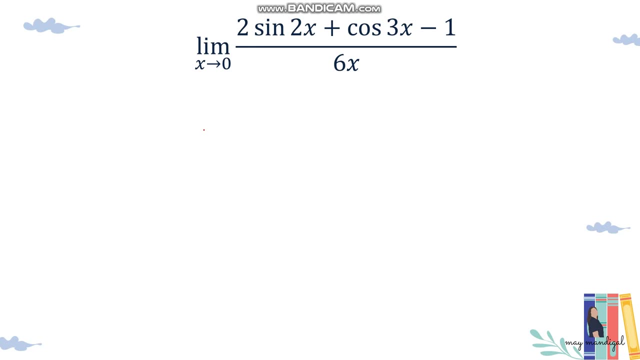 2 over 6 times 0, 0 or 1 over 6. so that will be our answer, or that is now the limit of our function. okay, another example: limit of 2 sine 2x plus cosine 3x minus 1, all over 6x. so in this case, as you can see, we have here two forms that can be. 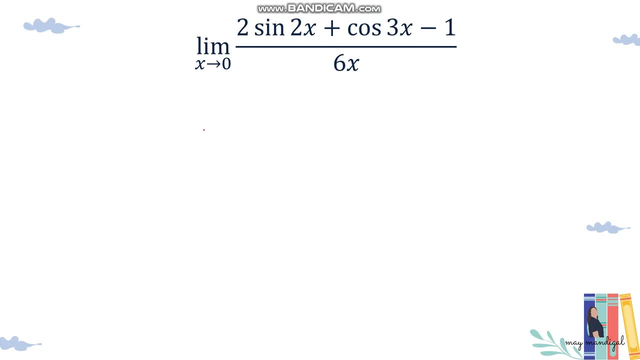 obtained later on. we have sine, we have cosine, so we should have sine x over x later in the form of sine x over x and also 1 minus cosine x over x. so this is our goal. we should have this later on. so what we will do here is: since there are two functions here, we can separate them into two. 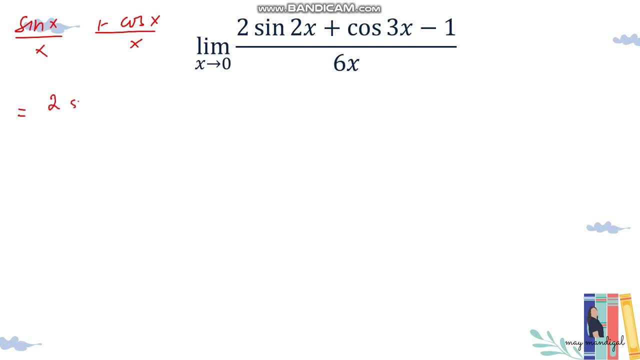 different fractions. so let's just write here: 2 sine 2x plus cosine 3x minus 1, all over 6x. so what we will do is we will separate the sine with the cosine and then they just have the same denominator, because this one is addition. so you have 2 sine 2x. 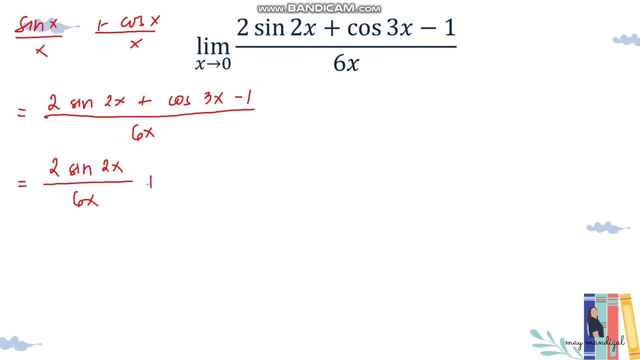 over 6x plus. and then we have here cosine 3x minus 1, all over 6x also. now we should rearrange this so that it follows this form: 1 minus cosine x. so what we will do is 2 sine 2x over 6x. 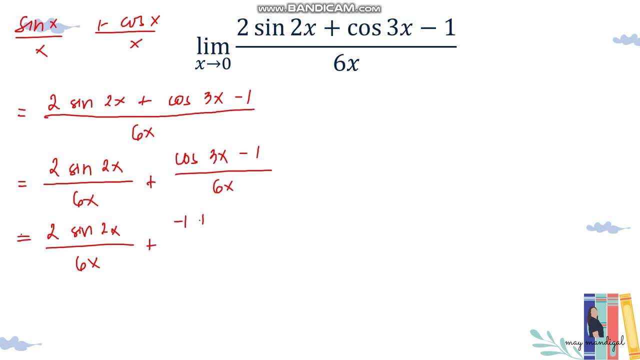 plus. and then we have negative 1 plus cosine 3x- all over 6x- and, like what we did a while ago, we factor out the negative 1, and then we have cosine 2x plus cosine 3x- all over 6x. 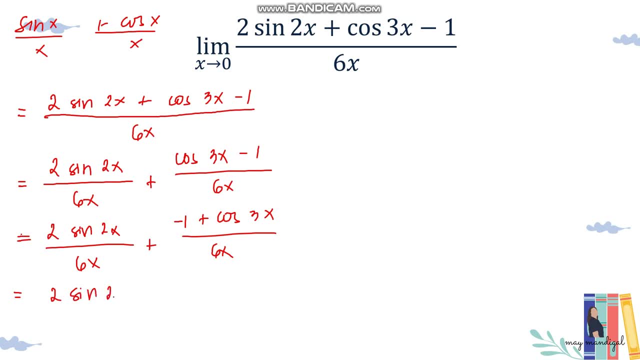 negative 1. so let me just write it like this, so in shortcut. so in short, this will be negative and then 1 minus cosine 3x. so this is just the same as what we did in the previous example. so you can refer to that. now we have here these two functions. what we will do is we have to just change them. 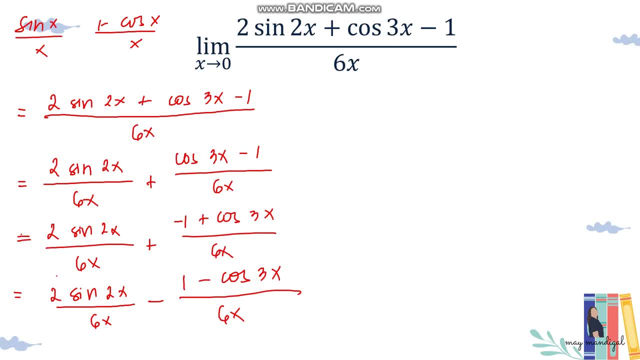 into similar numbers. so here for sine. so we the denominator here must be 2x. also for the cosine the denominator must be 3x. so what we will do is we will multiply them with two different values. so we have 2 sine, 2x over. 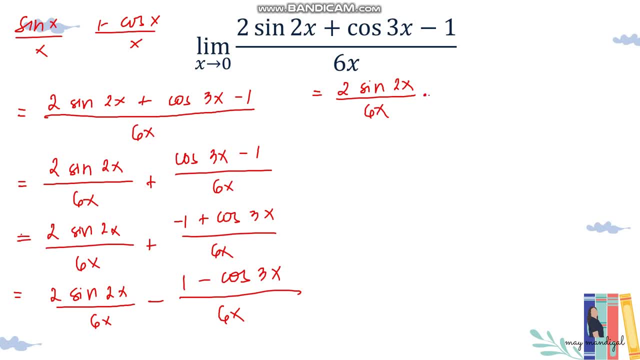 sine x. we will multiply this by 2 over 2. now why 2? like what i've said in the previous example, you have to use- or you can use- the coefficient of sine 2x and you can use the coefficient of sine 2x. 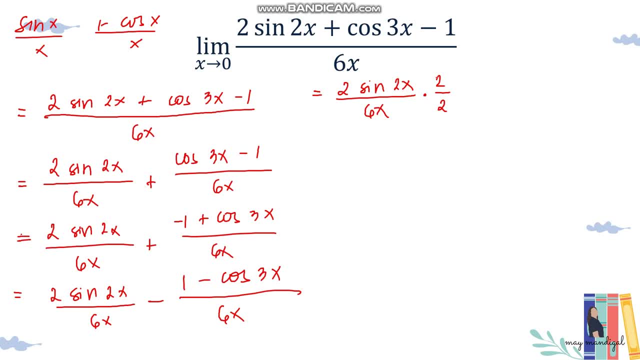 in the numerator and then use it to multiply the numerator and the denominator. so there, so what we will do is like that, and then we will also multiply the other side. so this one is 1 minus cosine, 3x over 6x, and then let's multiply it with again. 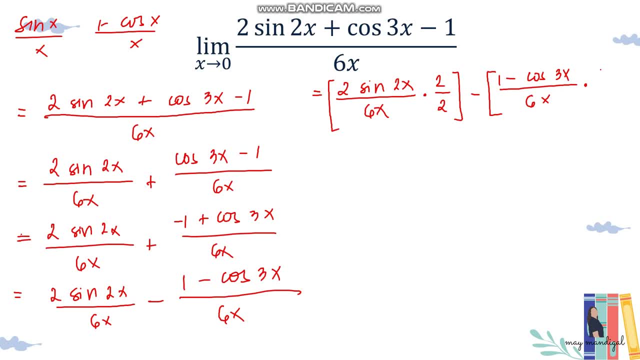 we're getting the numerator over the denominator and then we're getting the denominator over the or the coefficient of the numerator, so that's 3 over 3. and then let's simplify this. so we have 2 times 2 times 2. you can multiply, if you want. so 2 times 2 is 4, and then sine 2x. 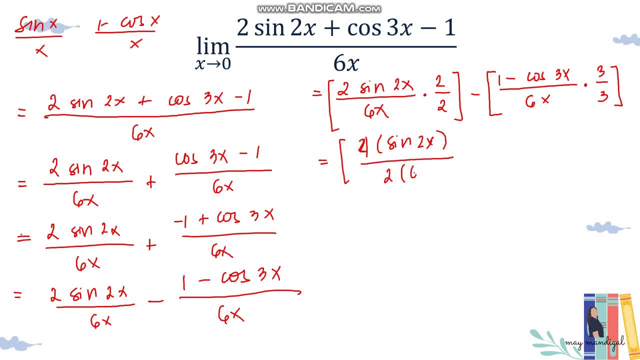 all over. then let's write here: 2 times 6x minus, and then this one is 3 times 1 minus cosine 3x, all over 3 times 6x. and then, like what we did in the previous example, let's interchange the values so that we can have the similar denominators. so we have here 4 and then 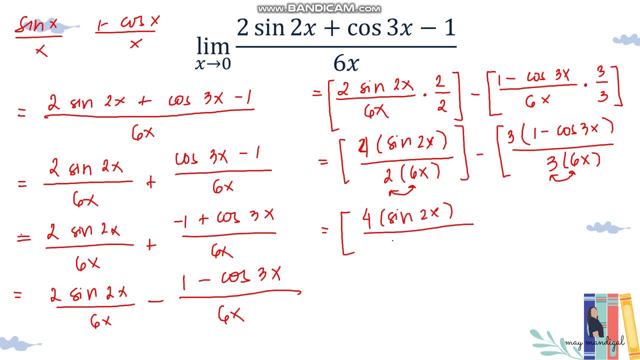 sine 2x over, and then this will become 6 times 2x minus. then this one is 3: 1 minus cosine 3x over 6 times 3x. so we now have something like this. so what we will do next is we can uh, remove the 4- 6 and the 3- 6 here. so by writing it and 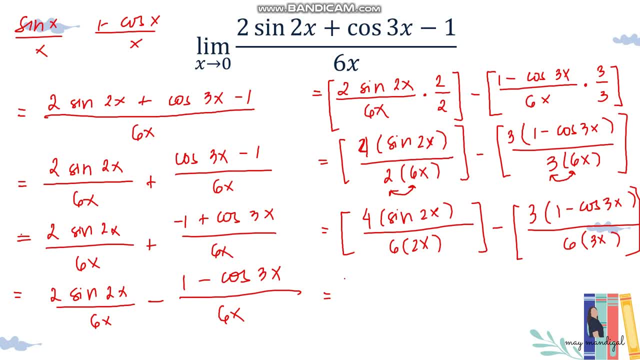 separate fraction. so we can also simplify: 4 over 6 is uh, two-thirds, so two-thirds, and then we can write two-thirds times. and then let's write sine 2x over 2 x minus. we can also simplify this. so 3 over 6 is 1 half times 1 minus. cosine 3x over 3 x. 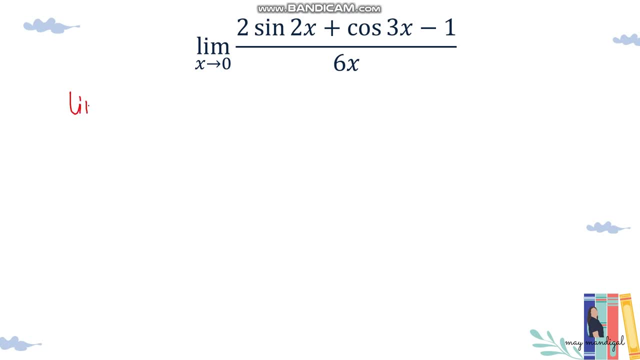 so after that we can now identify the limit. so let's write here limit of. and then we have the two-third times sine 2 x of the denominator and thenark form of each fifth, which is the sum of the x over 2x. and then we have there minus, uh, one half times one, minus cosine 3x over 3x. 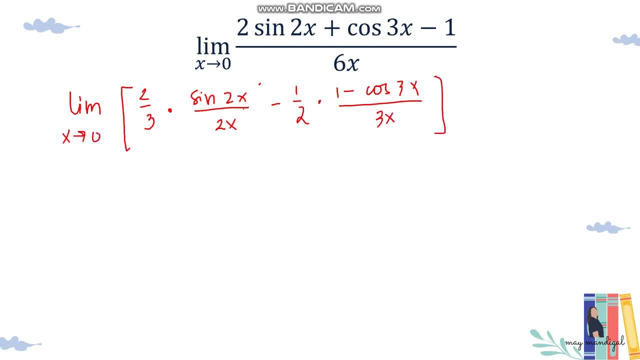 as x approaches zero. now if we substitute zero here, so it will be indeterminate also in this one. so that means we can apply, we can still apply the values for the special limits. so let's now identify the limit of this. so two-third, so we just have two-thirds here, times, and then for sine. 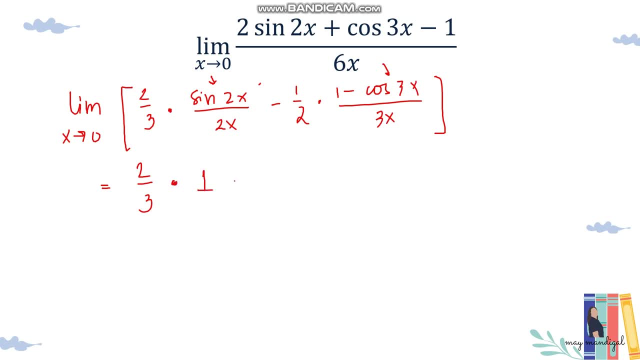 uh, the limit of that will be one minus, and then we have one half, and then this is times zero. okay, so, by the way, let's just put the grouping symbol like this there. so it's now like that. so we now have two-thirds times one is two-thirds minus one half times zero is zero. so 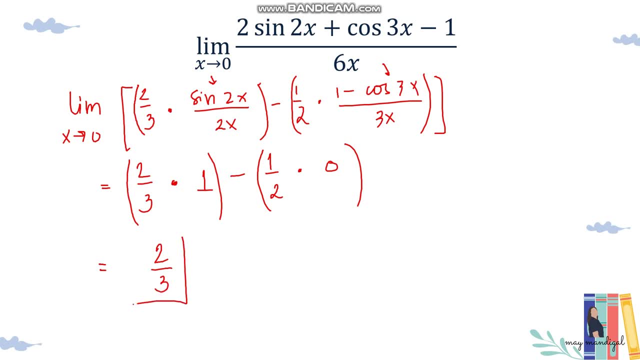 two-thirds minus zero. so in short, our final answer is two-thirds. so that is now the limit of our function as x approaches zero. and for our next example, let's say we have limit of e raised to 5x minus one, all over e raised to 2x minus one again. if we substitute zero to this, so that will: 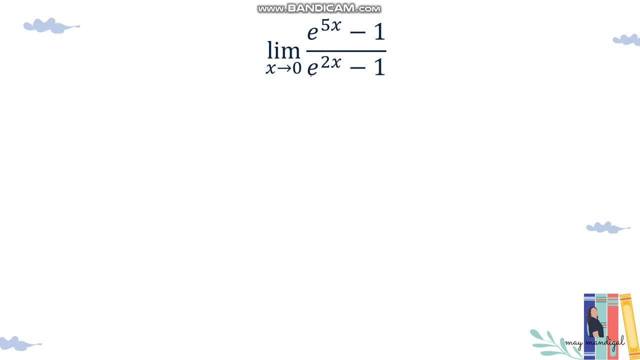 e raised to 0 minus 1 over e raised to 0 minus 1 or e raised to 0 minus 1, which is just equal to 0, same as with the denominator. so we will have an indeterminate value. now what we need to do: 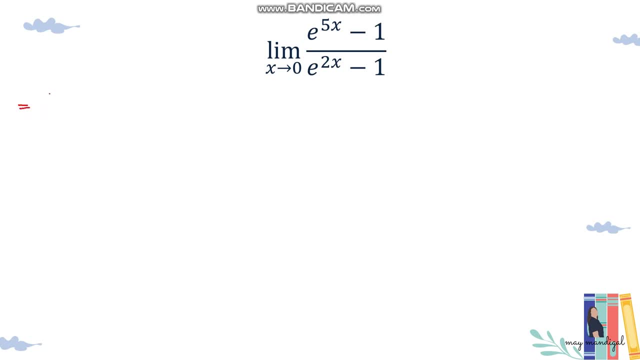 is to, of course, manipulate this. so let's just write here first the functions that we have. notice here that we have two different functions. so we have e raised to 5x. we also have e raise to 2x, e raised to 2x, e raised to 2x. 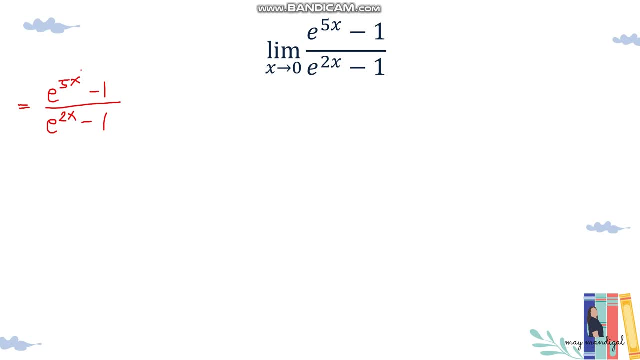 we also have e raised to 2x. so this means we will be having two sets of functions and, as you can see, one is in the numerator, the other one is in the denominator. so that means we have- we will have e raised to x minus 1 over x and 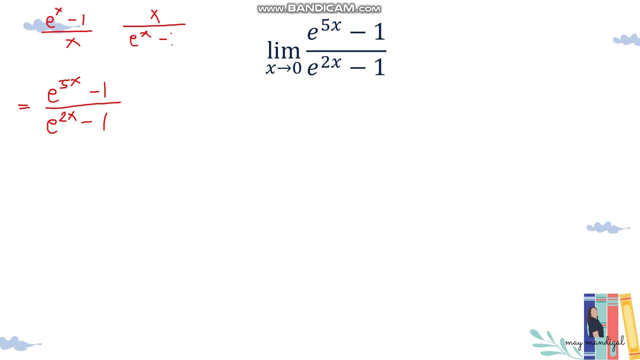 then the other one is x over e raised to x minus 1. so our goal here now is to separate this two so that we can come up with these forms. so if we will write here, let's write here the goal or our goal. so we have here e raised to 5x minus 1. so that is the first function or first expression. 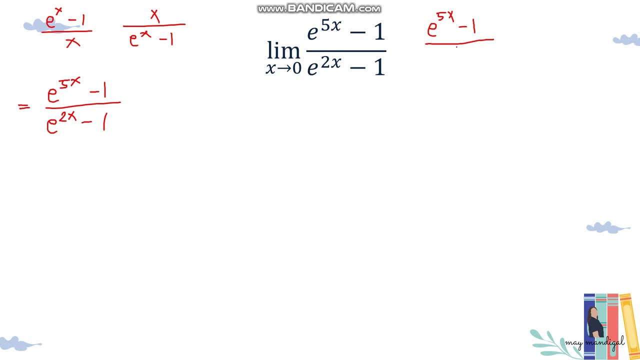 and for us to use the special limit or value of the special limit, the denominator must be the same with the exponent. so we need to have 5x as the denominator of e raised to 5x minus 1 for the second expression. so we have in the denominator e raised to 2x minus 1. 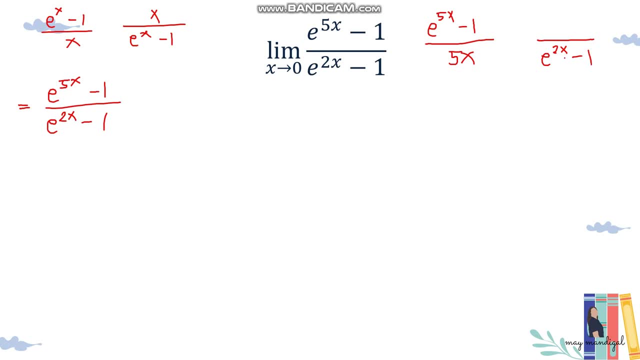 to use the limit, the special limit, the numerator here must be the same as with the exponent of e, so that is 2x. so our goal in manipulating this function is for us to arrive at these two functions here so that we can apply the values of the special limits now. in order to do that, 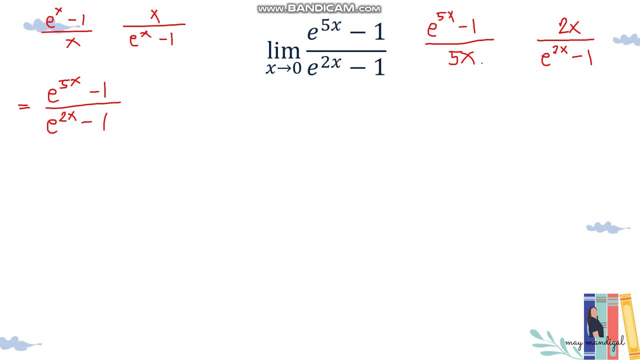 we have to multiply our function to certain terms or values. so what are the values that we have to multiply here? since we need 5x in the denominator, so we have to multiply this whole function, both the numerator and denominator, by 5x, and by 2x as well, because we 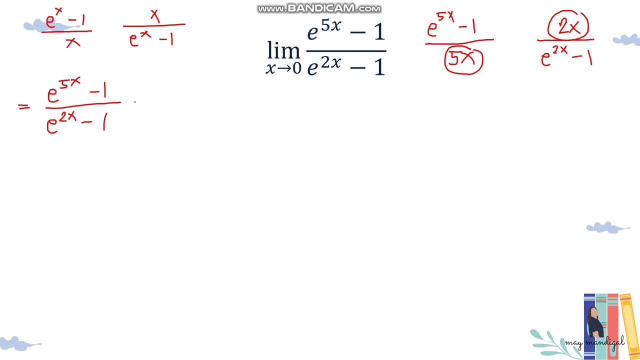 need it for our second function. so that means we have to multiply this by 5x over 5x and also 2x over 2x. now why again, we have to multiply both by 5x over 5x and 2x over 2x is because we need these terms in the 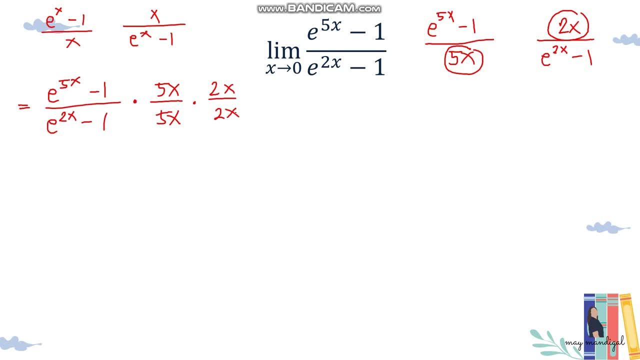 numerator and denominator of our function, so that we can apply the limit laws, so, or the values of the special limit, so what we will do here now. next is now, since we were multiplying this, that means we can again interchange the positions. since we are just multiplying, the terms are commutative. 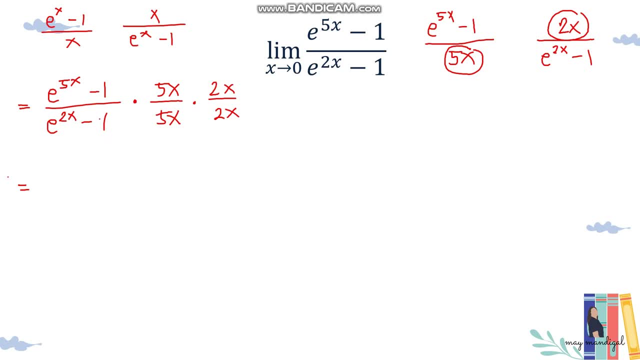 they will still arrive at the same value. so we have to multiply this by 5x over 5x and 2x over 2x. so to obtain this, this first function, right here, the denominator of this must be 5x. so what i will? 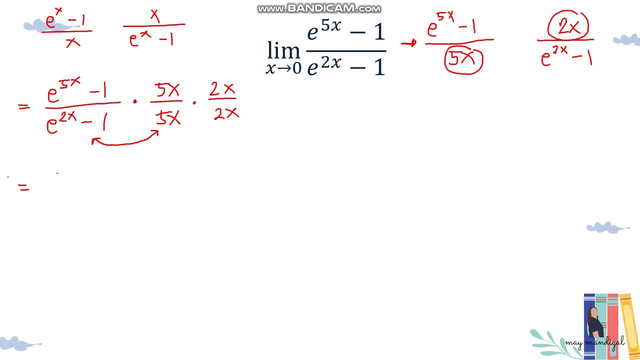 do is i will just interchange the two, so we will have e raised to 5x minus 1 over and then change it to 5x. then times now the denominator of 5x here becomes e raised to 2x minus 1, and then we. 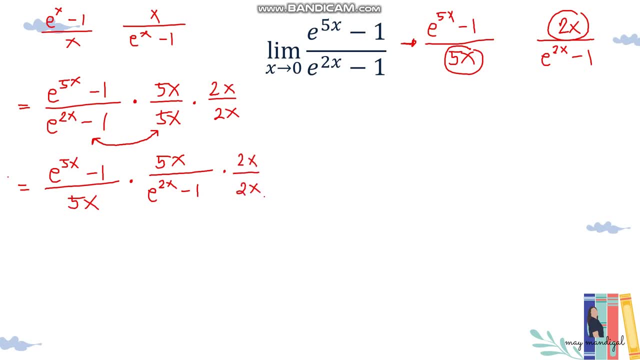 still have 2x over 2x here, so we have to multiply this by 5x over 5x and 2x over 2x over 2x. okay, so again, what we did is we just interchange the denominator of the first fraction to the. 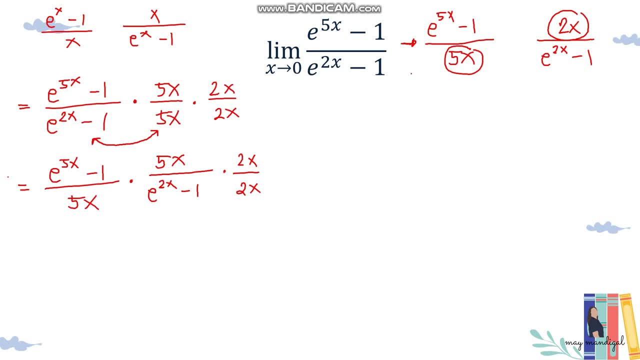 denominator of the second fraction, so that we can obtain this first goal. for us to obtain this first goal, which is this fraction right here now, in order for us to have this function, we need to change the numerator of the second fraction. so to do that, all we have to do is to interchange. 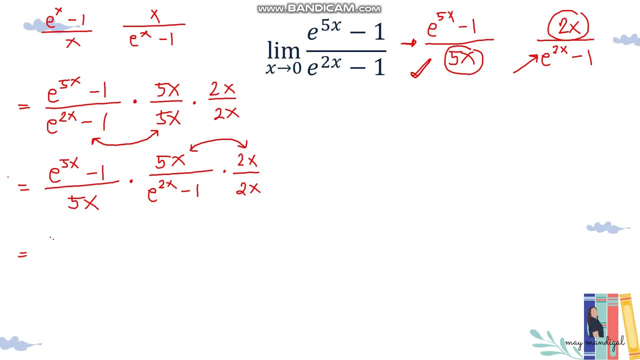 the denominator of the second fraction, and then we have to multiply the denominator of the first fraction and now to use the function we have to do is with 2 times times, and so we will have e raised to 2x and 5x. so what we will have here is e raised to 5x minus 1 over 5x times, and then change. so 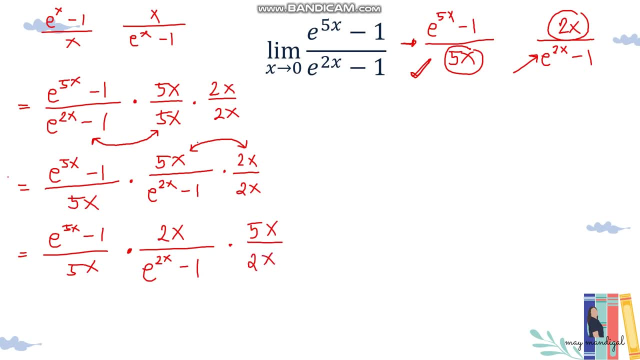 this is now 2x over e, raised to 2x minus 1 times, and then we have 5x over 2x. okay, so what we did? we interchanged the two and we're able to get this function. so, since we were able to obtain our goal, we can now apply for the second function. 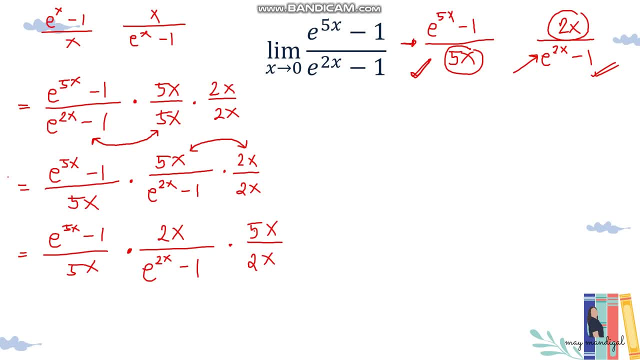 the values of the special limits. so, by the way, this x here can be cancelled. so what we have here is just 5 over 2. so let's now get the limit of that. so we have here e raised to 5x minus 1 over. 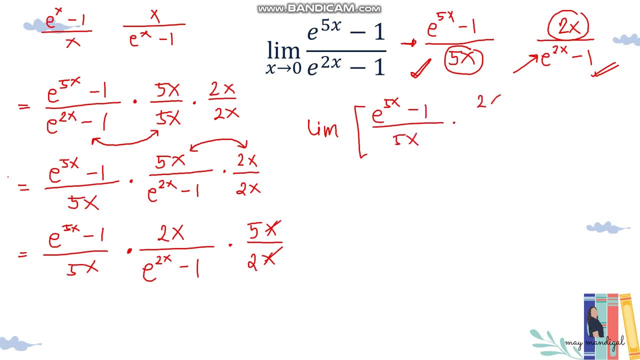 5x times 2x over e, raised to 2x minus 1 times 5 over 2. now to check: by the way, this one is x approaches 0. so if you substitute 0 to these two functions here, it will still be indeterminate. 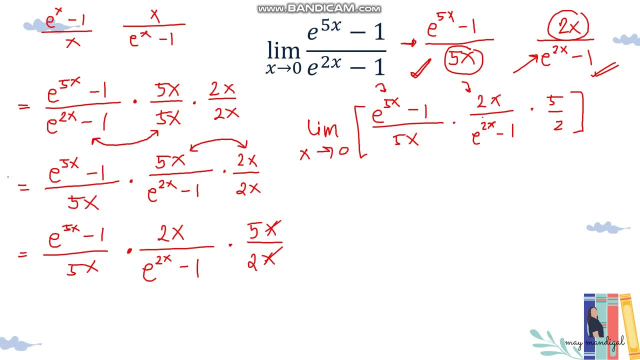 but since we now have same numerator and denominator, or the denominator of this is the same as with the numerator of e, the numerator of this is the same as with the denominator of e. therefore we can use the values of the special limit. so, for e or for this form, the value of the. 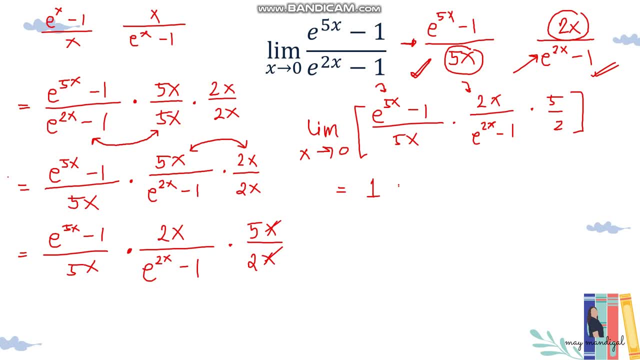 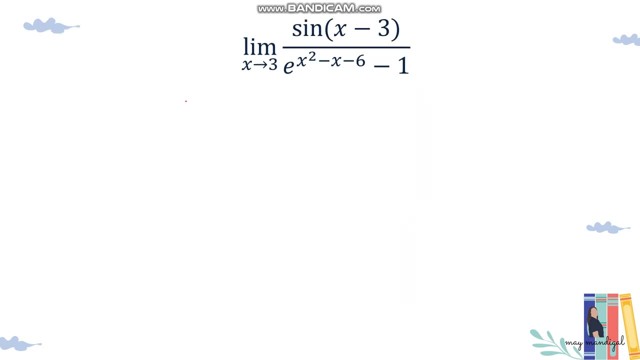 limit is 1, so another one is also 1, and then we have 5 over 2. so if we simplify that, therefore, our limit now is 5 over 2. so that is the limit of our function. and for our last example, limit of sine x minus 3, all over e raised. 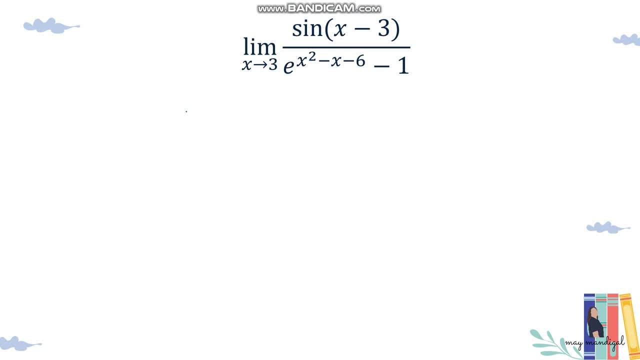 to x squared minus x minus 6 minus 1, as x approaches 3. now if you will substitute 3 to this function, so you will get sine of 3 minus 3, 0, so that is just 0. here you will get 9 minus 3 minus 6, which is again 0, so it will be indeterminate as well. 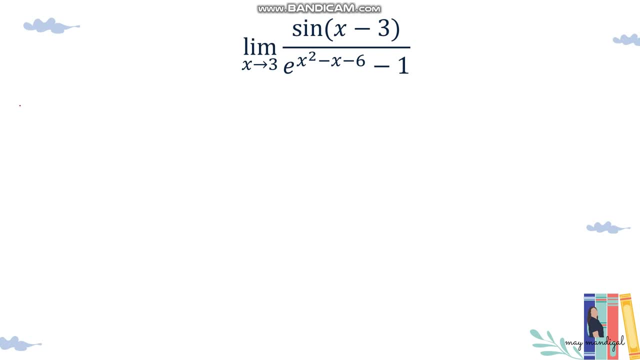 so that means we have to manipulate this equation. so let's just write here first: sine x minus 3 over e, raised to x squared minus x minus 6 minus 1. what we will do here is we have to observe what are the forms that we can obtain from this set. 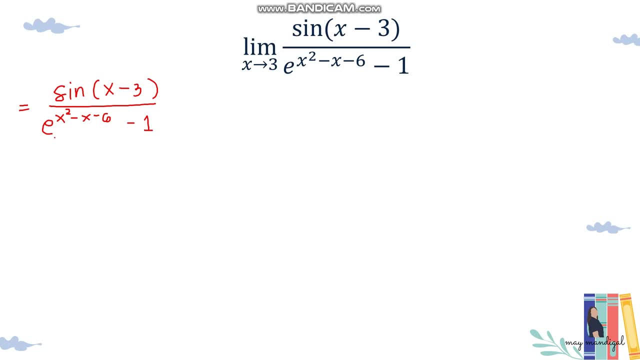 of function. so, as you can see, we have sine and then we also have e here. so that means we should have sine of x over x, since again because of the sine, and then for e, since e is in the denominator. so that means we should have something like x over e, raised to x minus 1. okay, so this is. 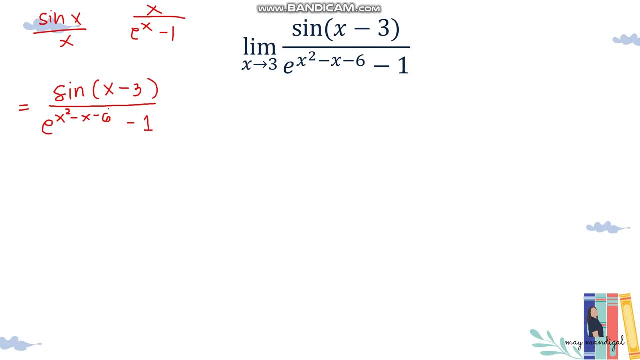 the forms, or these are the forms that we should have later on. now, how are we going to do it? so we have to separate this, so let's write here first the goals, or our goals. so, since i need sine x over x, but since it's x minus 3, so we should have sine x minus 3. 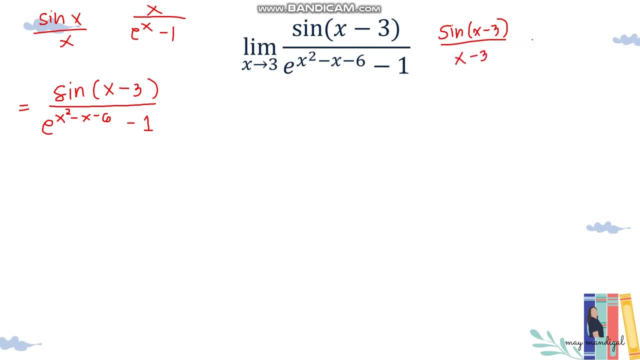 over x minus 3. and then the other one is: we have e raised to x squared minus x minus 6 minus 1, so the numerator should be x squared minus x minus 6, because the numerator must be the same with the exponent of e. okay, so this is our goal, so 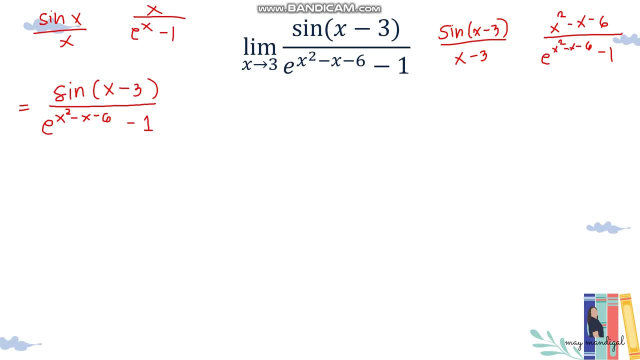 we should have this later on. now, how are we going to achieve this? so what we can do is: we can multiply, since we need x squared minus uh, since we need x squared minus x minus 6 and x minus 3 in this function. so we have to multiply this. but what are we going to multiply? um, as you notice, x minus 3 is. 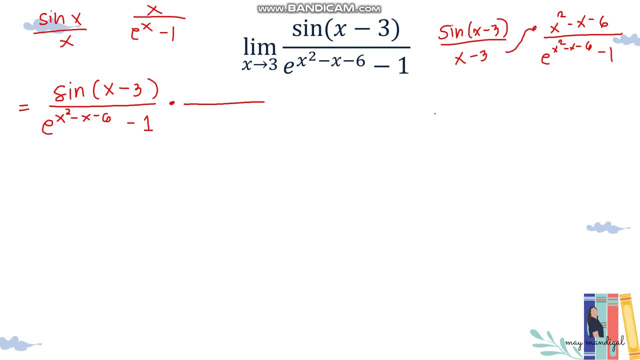 actually one of the factors of x squared minus x minus 6. okay, so no need to multiply this function by both x squared minus x minus 6 and x minus 3, so we will just multiply it with x squared minus x minus 6 again, because x minus 3 is actually a factor of this given trinomial. so later we will. 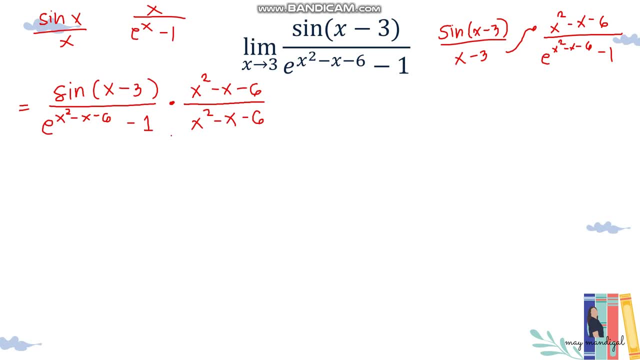 do something about it so that we can have x minus 3. so what we will do here is: since i need x squared minus x minus 6 as the numerator of this expression, so what we can do is we can just interchange these two so i have sine x minus 3, sine of x minus 3 over, and then 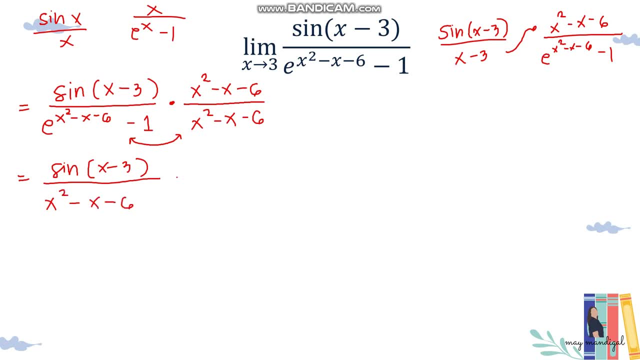 x squared minus x minus 6 times. and then i have x squared minus x minus 6 over e, raised to x squared minus x minus 6 minus 1. okay, so this second fraction that we have here, this one, is already okay because we're able to get. 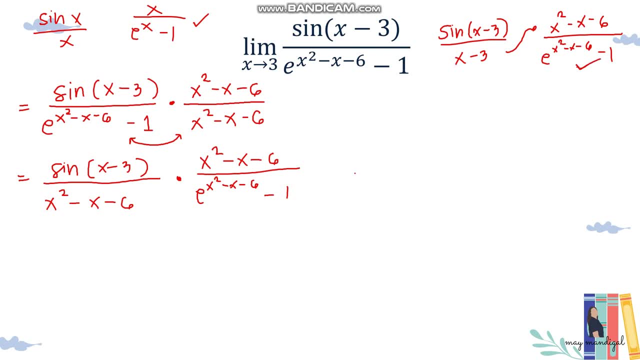 our desired function or form. so that's already okay. however, we still have to manipulate the first one, because what we want is the denominator should be x minus 3, but again, x minus 3 is one of the factors of 4, so what we can do is we can factor that, so sine of x minus 3, over factoring. 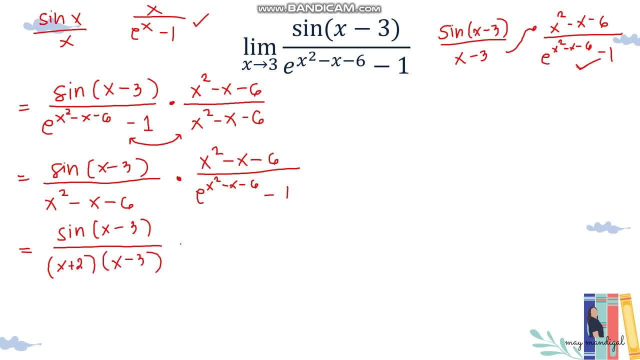 x plus 2 and x minus 3, and then just copy this one, x squared minus x minus 6, over e raised to x squared minus x minus 6 minus 1. okay now, since we have here now this one, all we have to do is to: 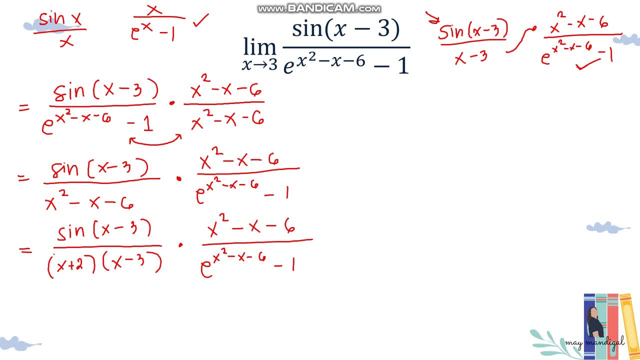 separate it, write it in a separate fraction and also the x plus 2 in the denominator, so that will be 1 over x plus 2 times. and then let's write this function here and then we have x plus 2 over x plus 2 here, sine of x minus 3 over x minus 3 times. then x squared minus x minus 6 all over e raised to. 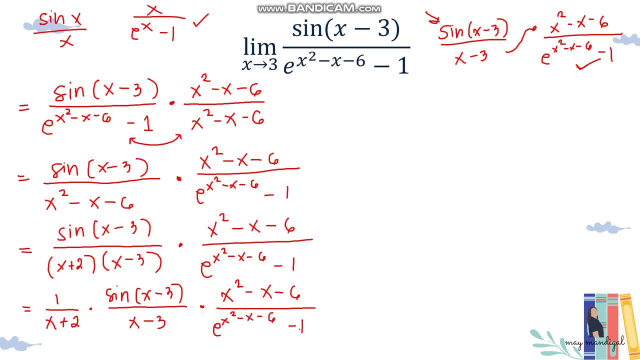 x squared minus x minus 6 minus 1. now that we obtained our goal, we can now identify the limit of this function. so limit of. and then let's just write here: 1 over x plus 2 times, and then we have the sine x minus 3 over x minus 3, and then times x squared minus x minus 6 over e raised to x squared. 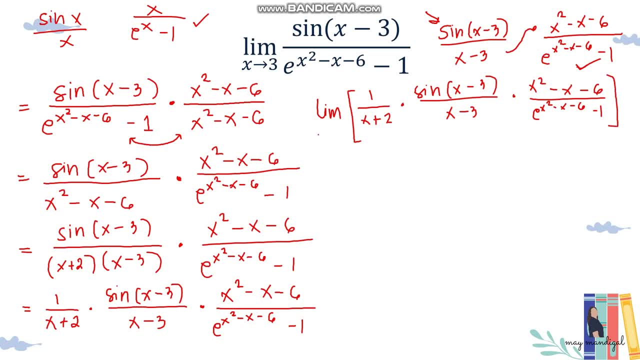 minus x minus 6 minus 1, as x approaches 3. now can we use the values of the special limits? this time x approaches 3. so, like what i've said a while ago, you can just substitute 3 to check if our functions here will become indeterminate. so if you substitute 3 to this, so sine of 3 minus 3, 0.